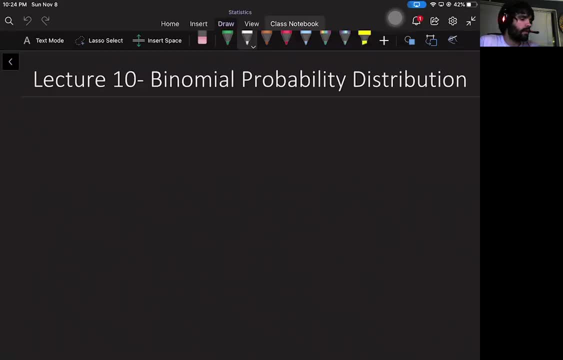 Hello class, welcome to lecture 10.. Today we're talking about binomial probability distributions, which have a very fancy sounding name, but they're going to turn out to just be like very special situation of these charts that we've been learning about. 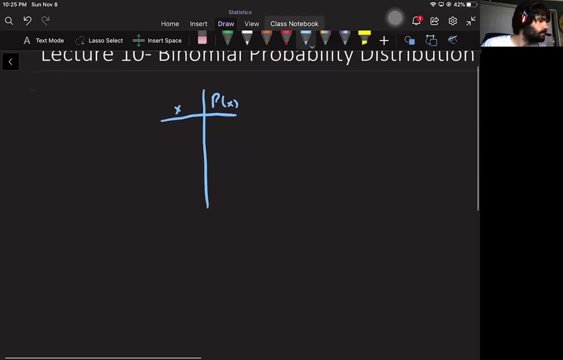 Okay, so let's just jump right into it. So we're going to, like, create a question And, from this question, talk about what we want to talk about. So let's think about situation like this: So consider a probability experiment where spare in, where there are only two outcomes. 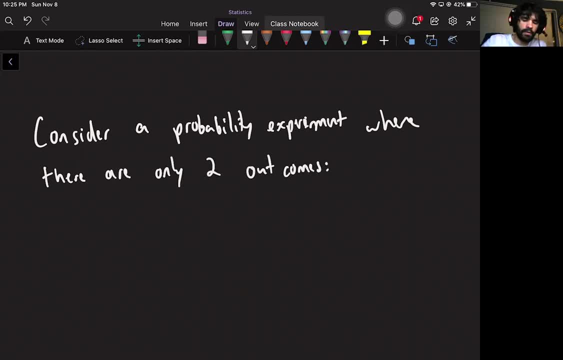 So two outcomes are always going to be called success or fail. Now it's up to you to decide what a success is and what a fail is, But that's always what it's going to be. So, for example, something like this I could like: shoot a free throw. 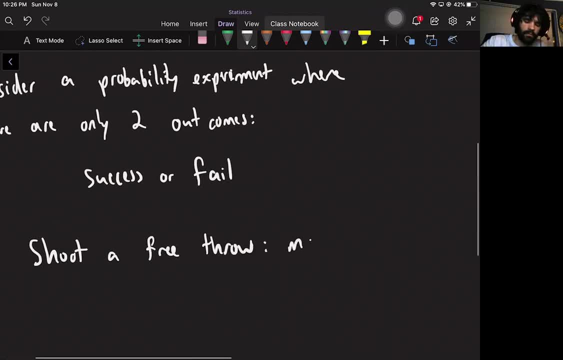 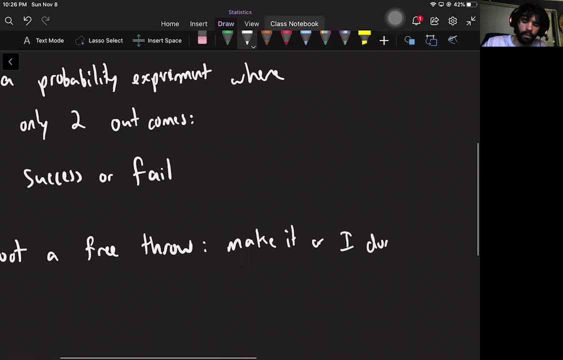 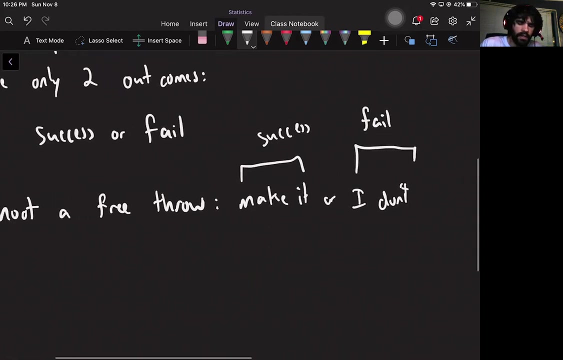 So then I either make it or I don't. So there are only two outcomes. Typically you would call that the success, Unless you want to be like really strange for some reason, and missing it you would call the fail. Notice that it's not necessarily a 5050 chance. Right, I'm very bad at basketball. 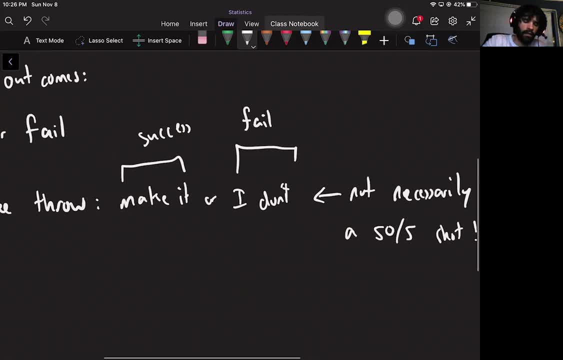 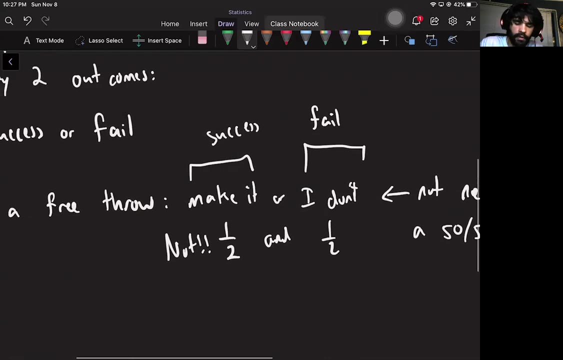 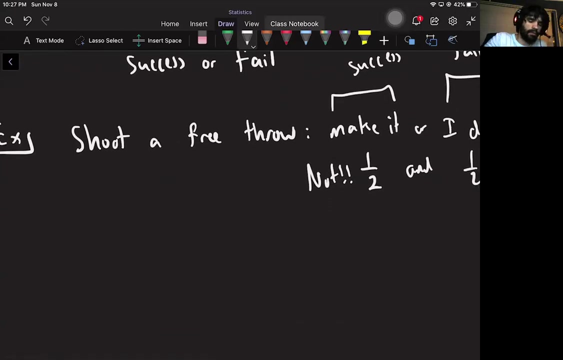 So it's not like. it's not like automatically one half probability of success And one half probability of fail. For me it would be very low probability of success And high probability of fail. it would not just be 5050. But there's lots of other examples. So some sort of like machine doing a task. 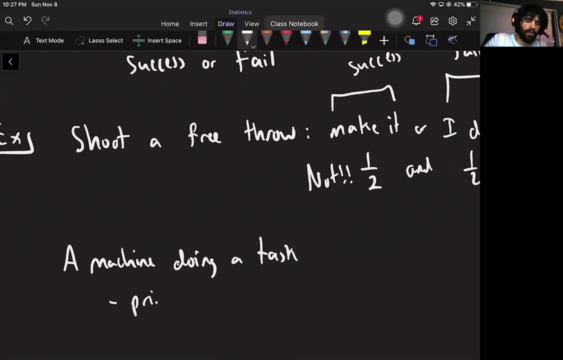 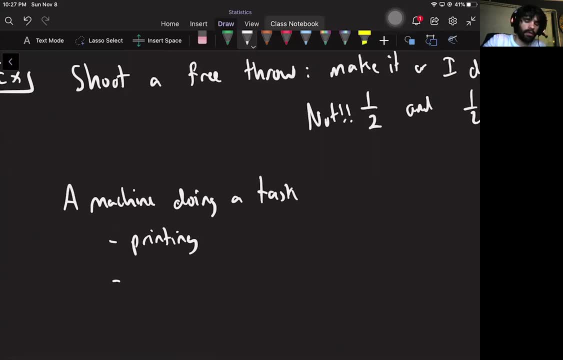 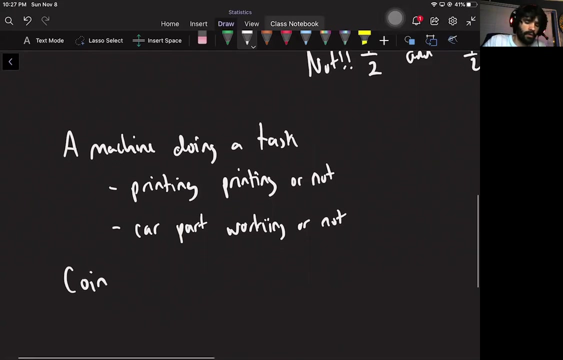 So like printing or something. So either the machine, the copier, prints or it doesn't, or a car part working or doesn't work, Stuff like that. So a lot of things can be thought of like this. So more familiar one that we've been dealing with: coin flips, So you could think of a coin landing on 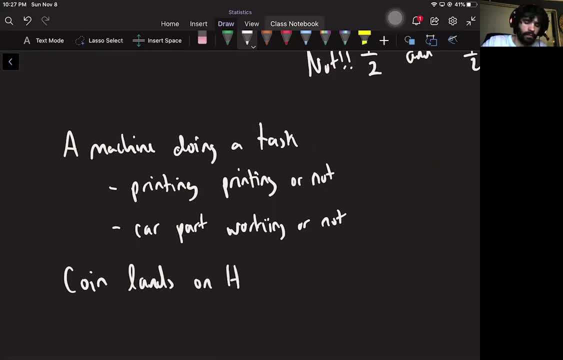 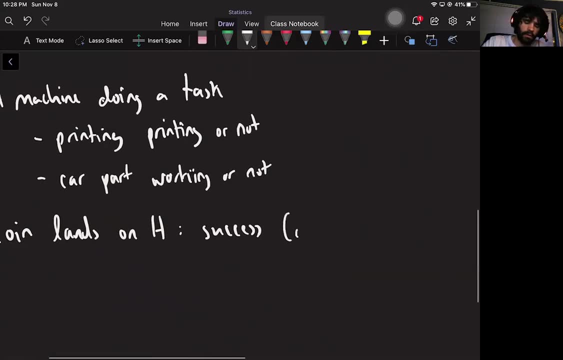 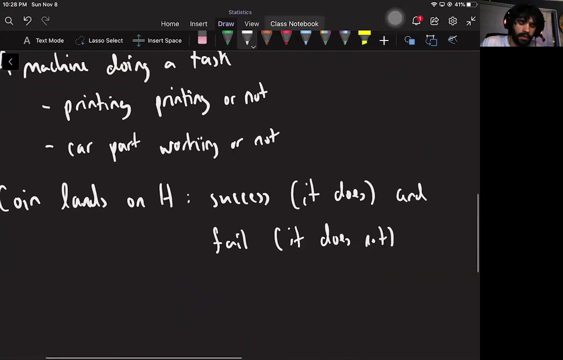 heads as a success And if it doesn't land on heads, then you call that a fail. So successes it does do that And fail would be that it does not. So this one is 5050.. The success and failure, both 50% chance, one half probability. but it doesn't have to be like that. 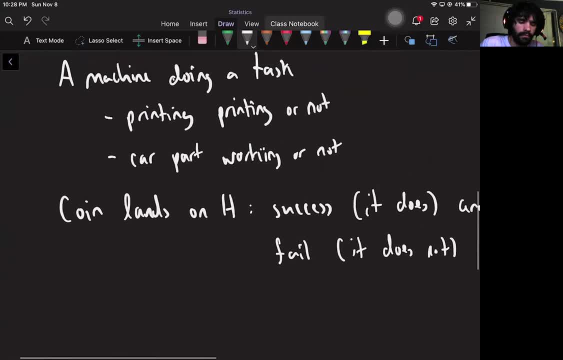 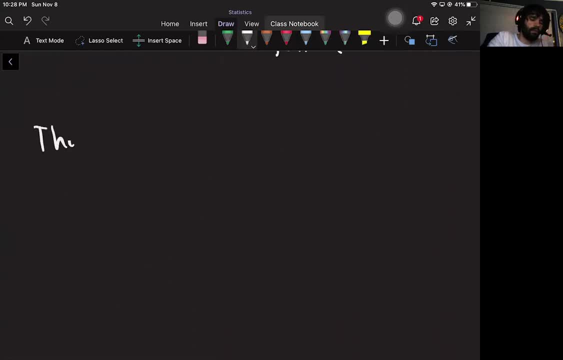 Ok, so what we do? we have our probability experiment with just two outcomes: success or fail. So then, whatever your experiment is, we repeat it some amount of times. Experiment So many times So you can pick that ahead of time. Okay. 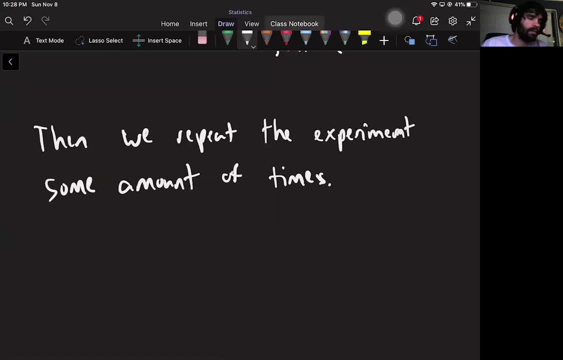 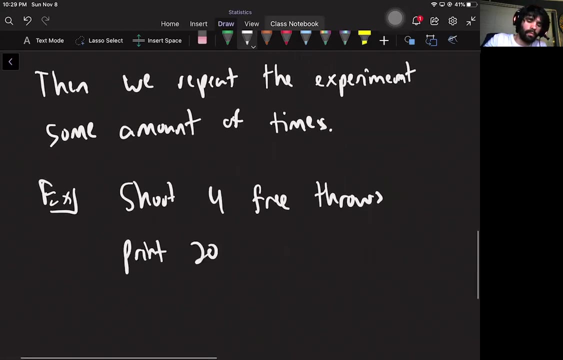 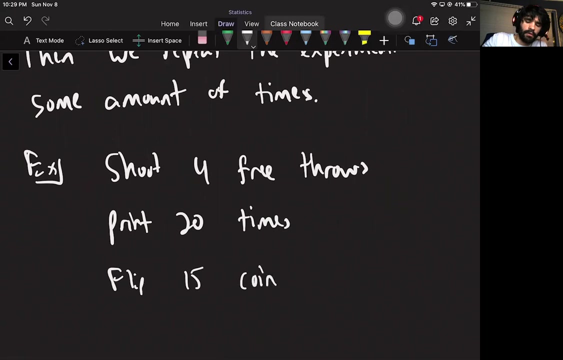 Does that help? Sure, Okay, like 10,, 30 times, four times, whatever you want. So I could shoot four free throws, for example, Or I could try to print 20 times, Or I could flip 15 coins. 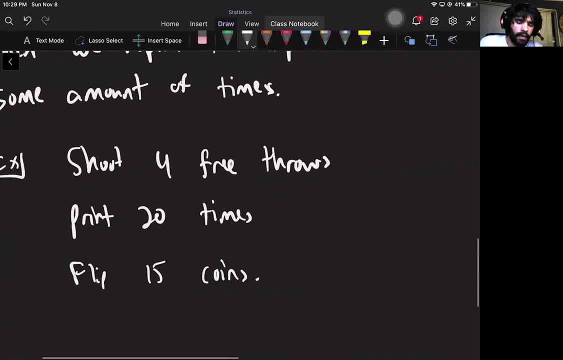 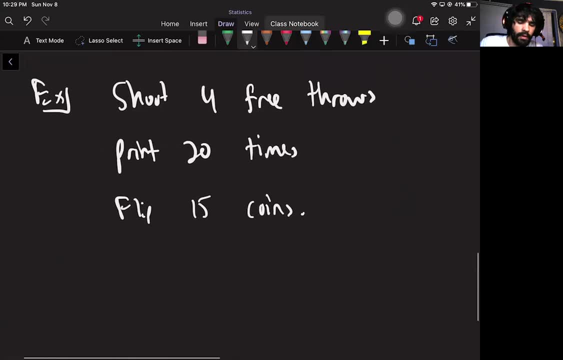 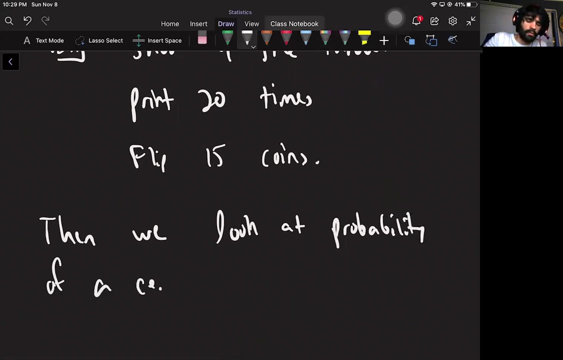 So then the idea is, each time I'm doing it I'm thinking about if I'm succeeding or failing, And then I wanna look at probability of that happening. Okay, so then we look at the probability of a certain number of successes. 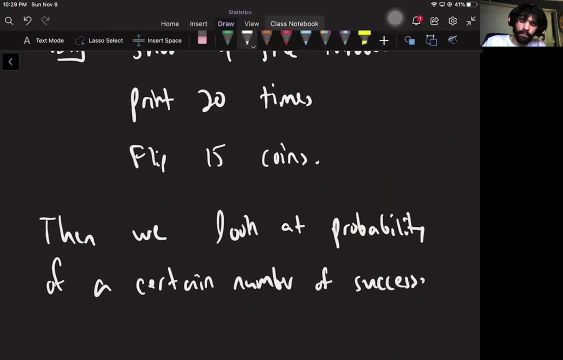 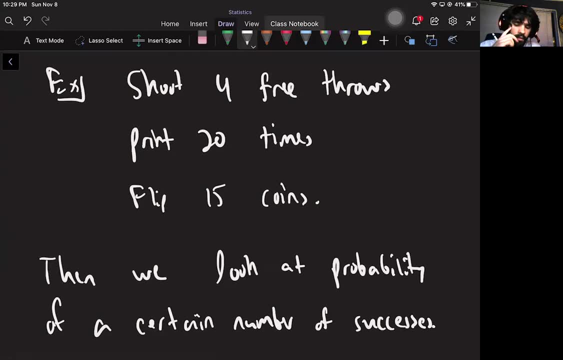 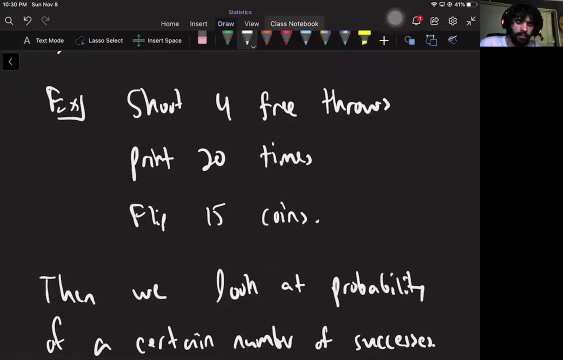 So if I shoot four, three free throws, maybe I wanna know what's the probability of making two, Or probability of making three Or one Or all four Stuff like that. If I print 20 documents, what's the probability that 15 of them actually print and five don't? 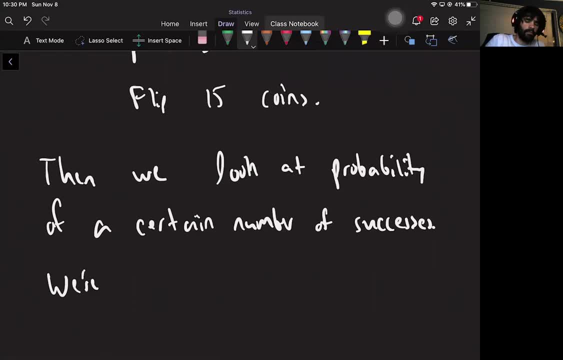 So the nice part is, we're gonna figure this out just by knowing the probability of one success. So we're- Let me write it like this: So we'll figure it out from knowing just the probability of one success. Okay, A single success, I should say. 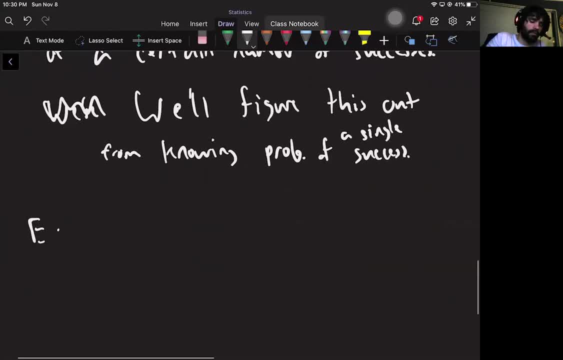 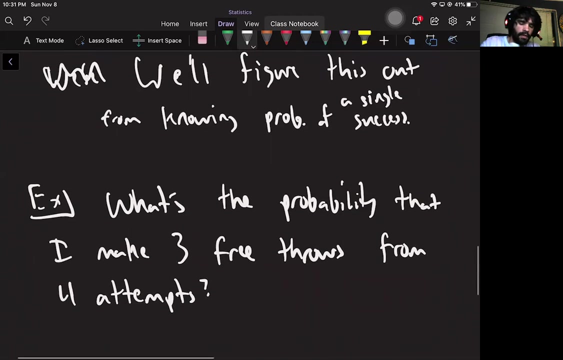 So let's do it with the free throw example. So what's the probability? Let's say that I make about three- three free throws from four attempts, And so when I say questions like this, I'm always gonna be secretly using the word exactly. 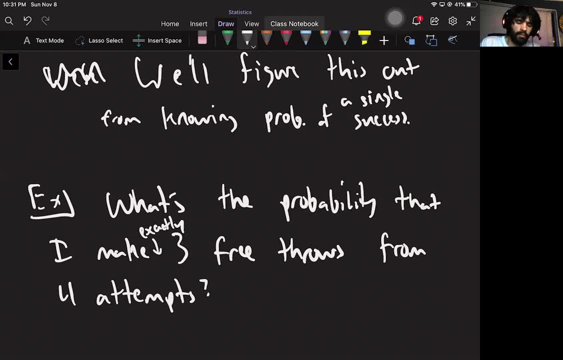 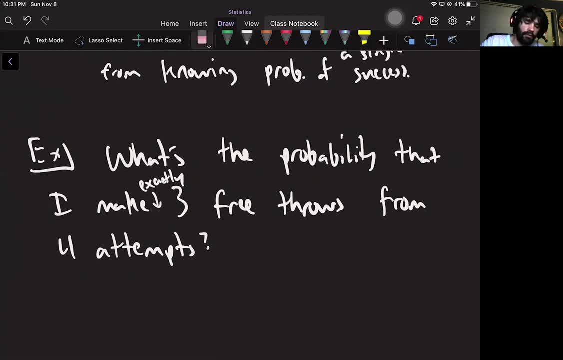 So exactly three free throws, not So four attempts, Or making all four does not count, Just exactly three. So what's the probability of doing this? if I gotta finish the question, If my probability of one success, Probability of one success, 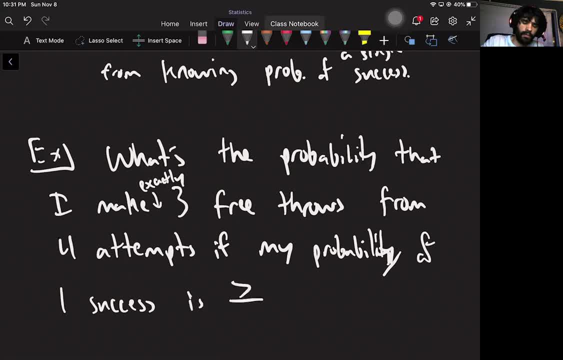 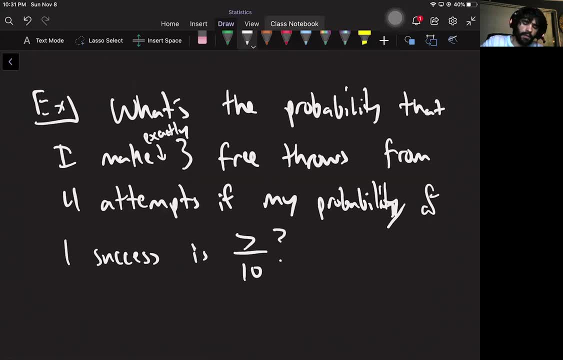 AKA making one free throw is I don't know. pretend I'm actually decent seven out of 10.. So if I know that, if I just do it once at any one time, my probability of making it as seven out of 10,. 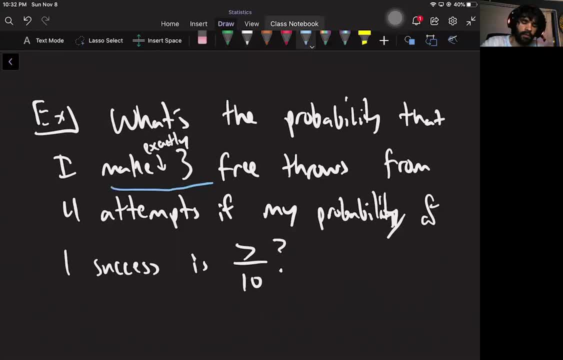 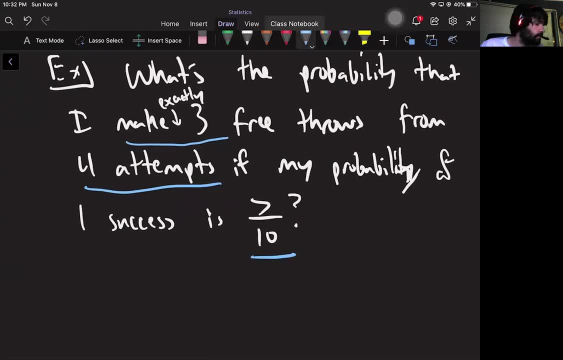 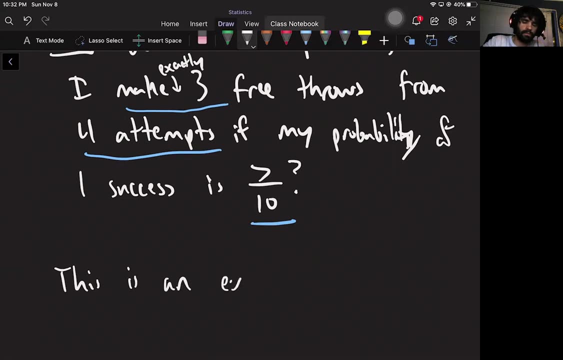 then, using that, what's the probability that I can make exactly three if I try four times? So these are the relevant pieces of information here. Okay, so this is an example of something called a binomial experiment. So let me say that is before we tackle this problem. 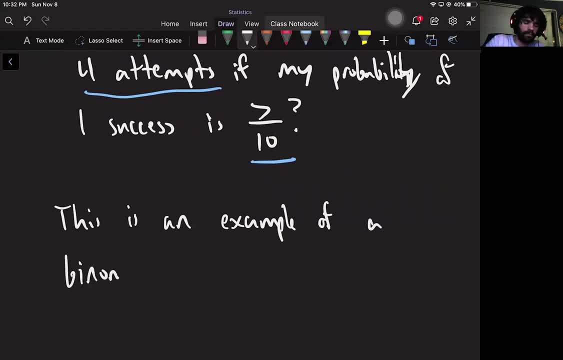 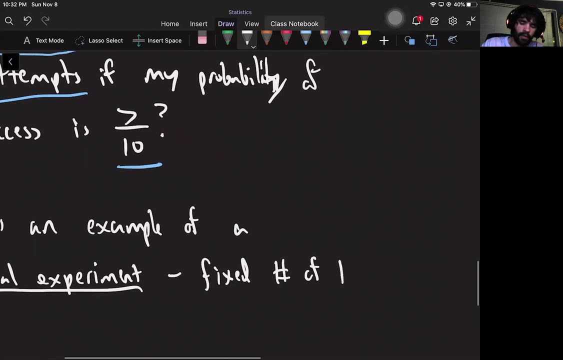 Binomial experiment. So what that means is that you have a fixed number of trials. that's how many times you do the thing. So in this case that's four, Because I'm trying four free throws. The answer is six Okay. 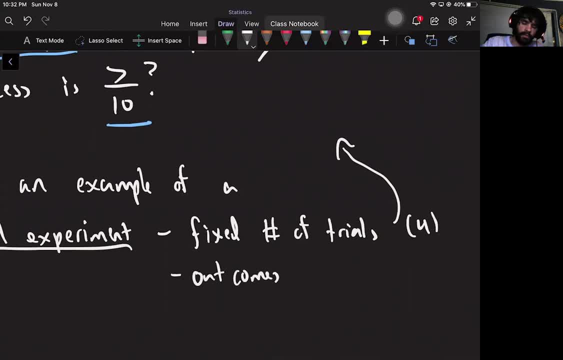 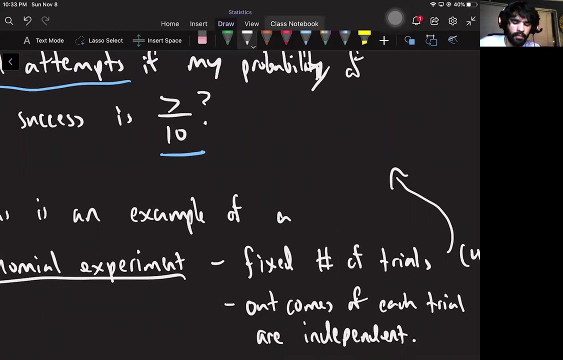 the outcomes are independent of each trial. so what does that mean? well, remember that independent. that actually means something important. that means that they don't affect each other. so what this is saying is: i have to assume that making one free throw or missing one free throw doesn't affect my chances of missing, or? 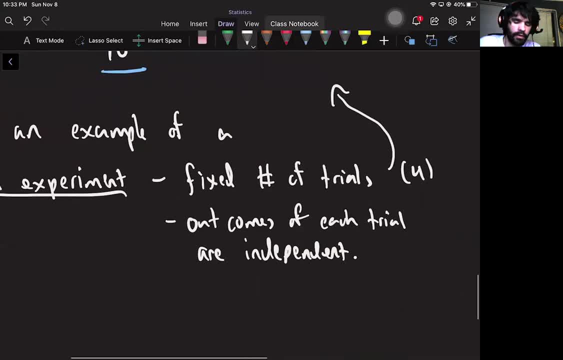 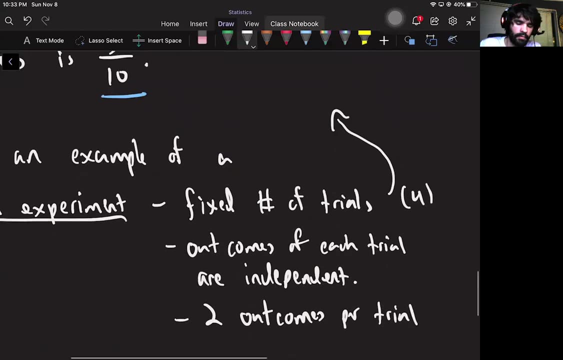 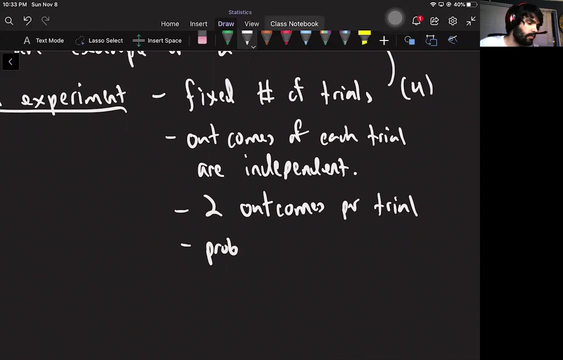 making the next one. they're independent of each other. any one throw does not affect a different throw um. and then there's got to be the two outcomes per trial, that's the successor or fail um. in this case it's making it or missing it, and the probability of success has to just stay the same per trial. 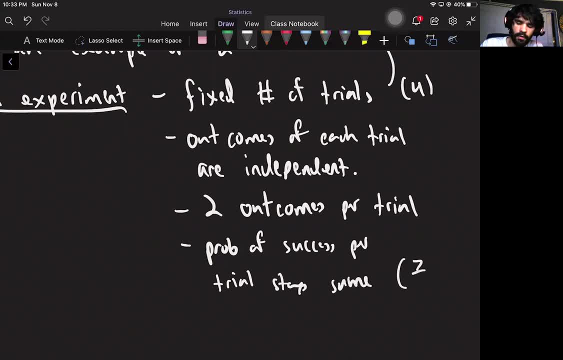 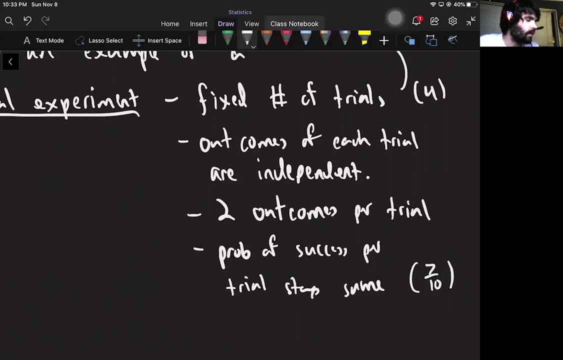 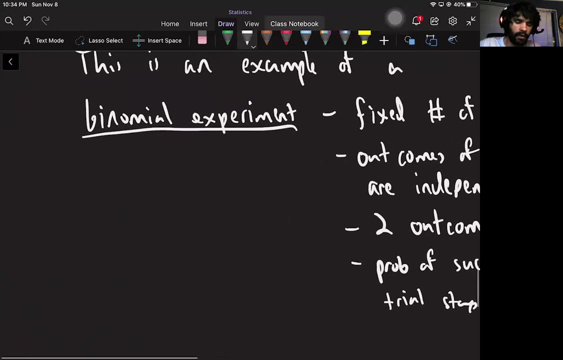 so in this case, each individual trial, the probability is always 7 out of 10.. okay, but this is. these are the four requirements to be a binomial probability binomial experiment. okay, so now what we're going to do is we're going to make a probability distribution dealing with 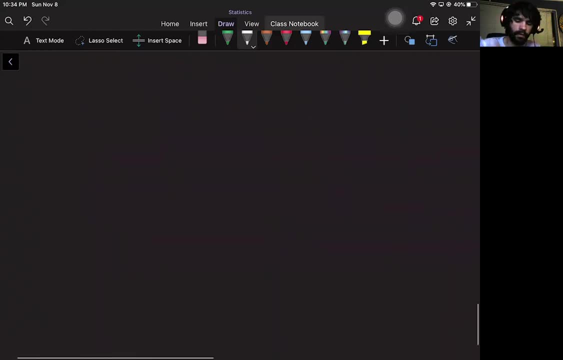 this situation. okay, so what does that mean? we need um, we need a random variable so we can make the meowstrahl probability distribution. that just means a little chart um, and to do it you have to have a random variable which can be a couple different numbers, as as those are what our little x's were last time. 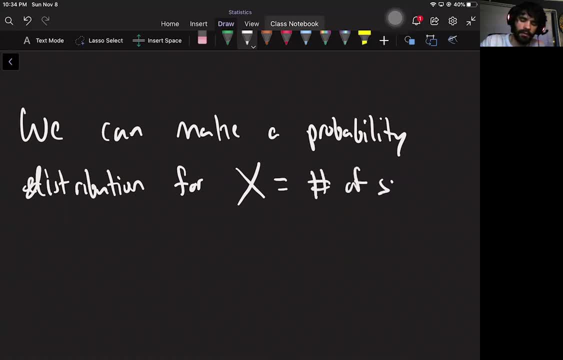 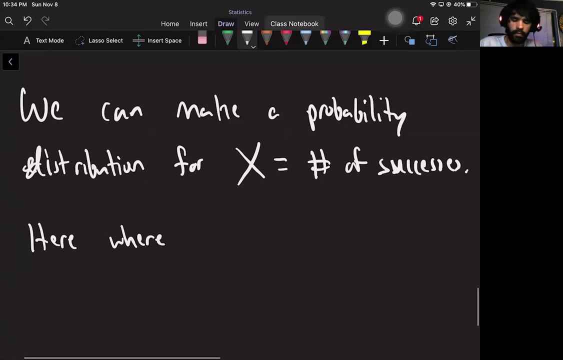 so. so our random variable is going to be the has to be a number, so it's going to be the number of successes. And so in this example, if I, if I try to make four free throws, that means I'm doing four trials. 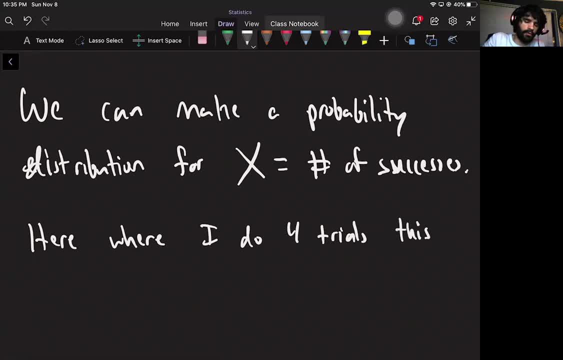 This means that my random variable can take which values? what can little x be? What What numbers can this be? Well, if I'm making, if I'm trying to four times, I can either make zero shots, I can make one, I can make two, I can make three or I can make all four. 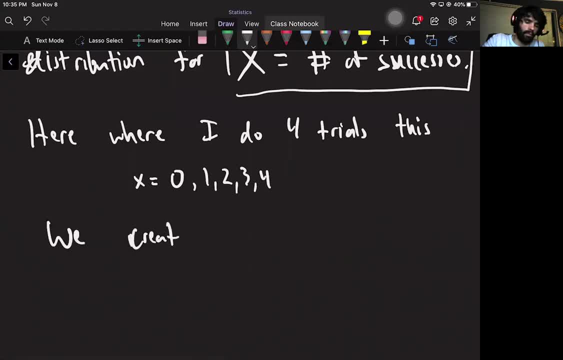 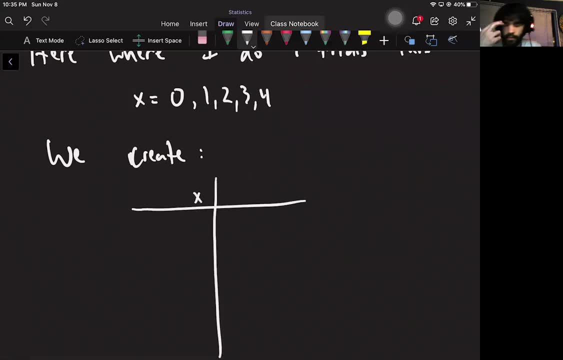 So then we create the probability distribution, where on the left side there's always this little x, which are the possible values That the number of successes could be. So since I'm trying four times, I can go from zero to four. 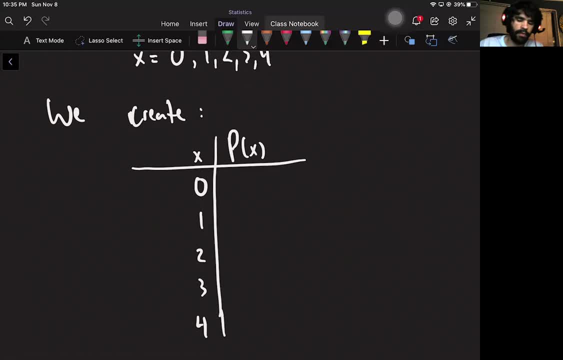 And then, next to each little x, is the probability of that happening. So So, again, just to remind you this, these numbers are not just randomly there. These represent the number of free throws. in this example, Three, three free throws. Three free throws made in four trials. 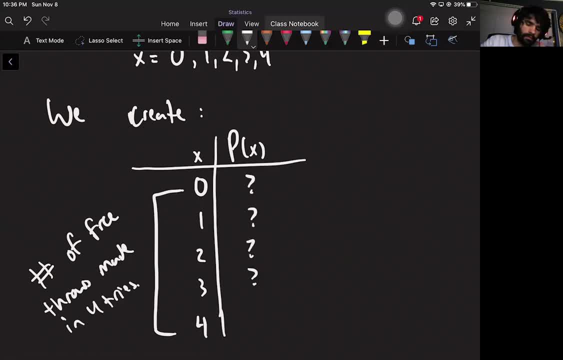 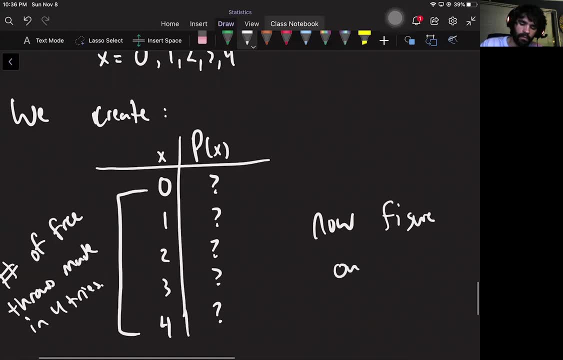 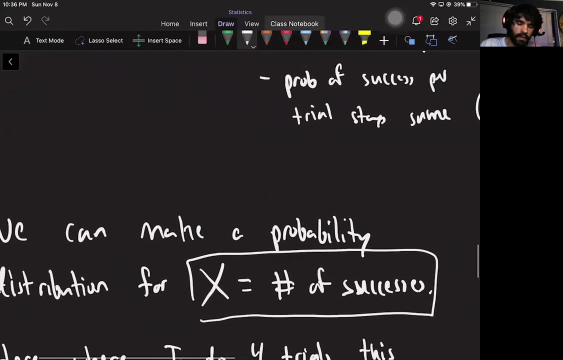 And then over here, we don't know these. we're gonna figure these out, So now we'll do that. Now notice that this third one here. that's what this question was asking about earlier. What's the probability that I make exactly three free throws from four attempts? 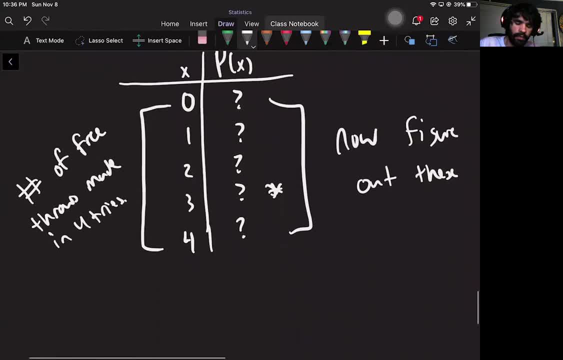 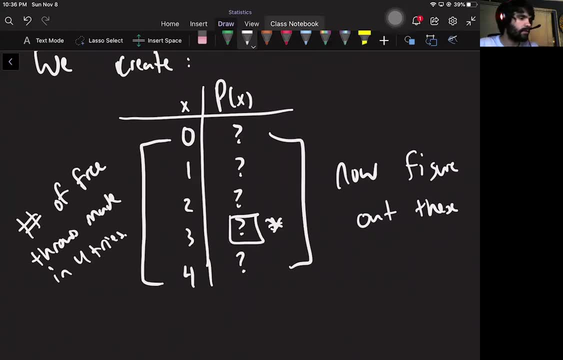 If my probability of one success is seven tenths. That's exactly what this is finding that, but now we're going to do all four Okay, and it's not so bad. The reason we're studying these particular kinds of probability distributions is because 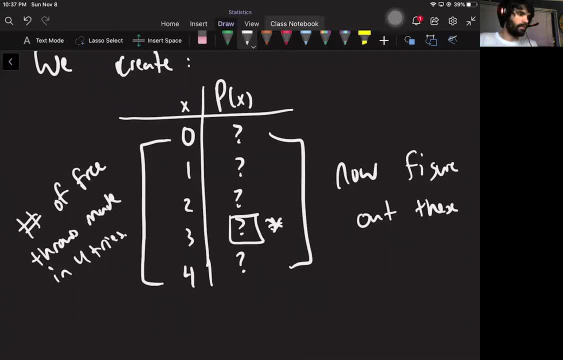 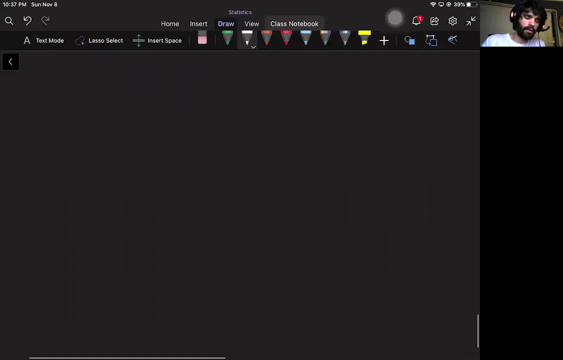 they are easier to deal with, And we'll see that right now. Okay, so so let's figure these out as our next goal. So to begin Figuring these out, first notice Something interesting that you might remember: if the probability of success is seven out, 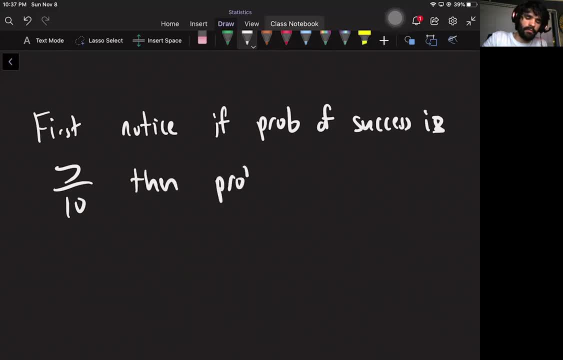 of 10.. Then, what's the probability of failure? Well, you either do one or the other right. So if probability of successes Okay, Okay, Seven tenths, That means probability of failure must be three tenths, because it's one minus seven. 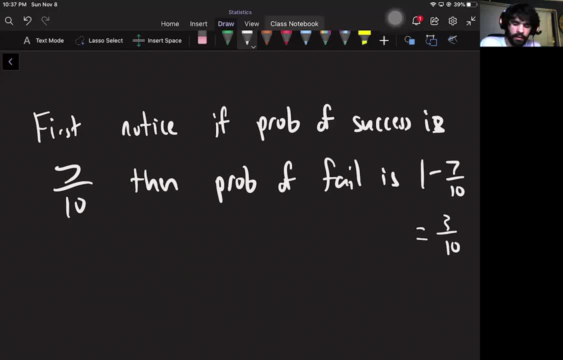 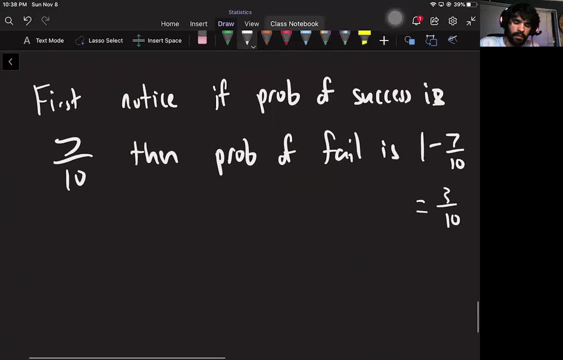 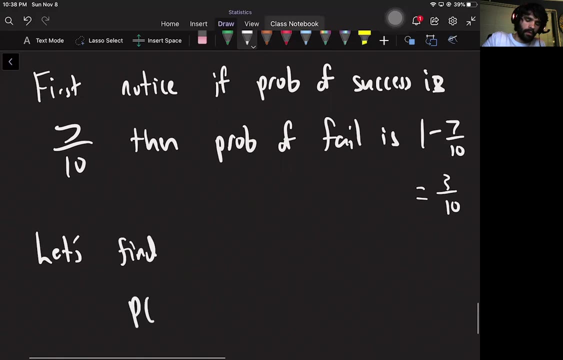 tenths. Okay, it's just like the rest of the probability, because it's got to add up to one, because something has to happen. Either you succeed or you fail. Good, So that's the probability of failure. So now let's start by finding this thing, which was the first one on the list, but just 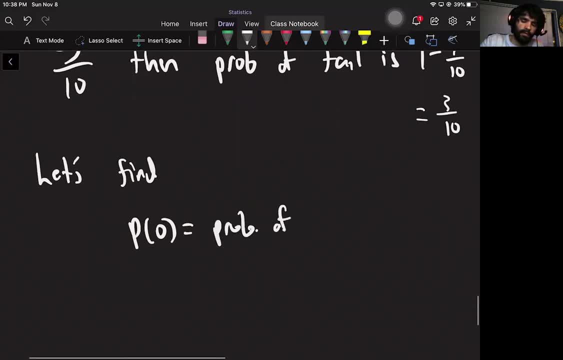 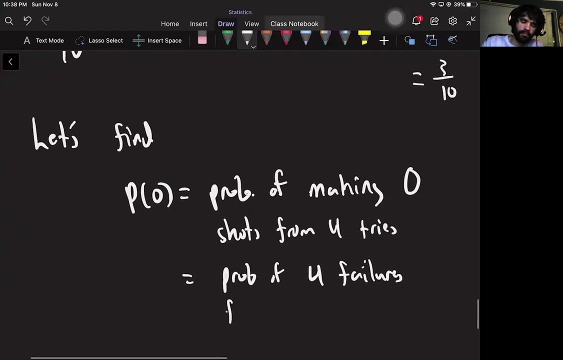 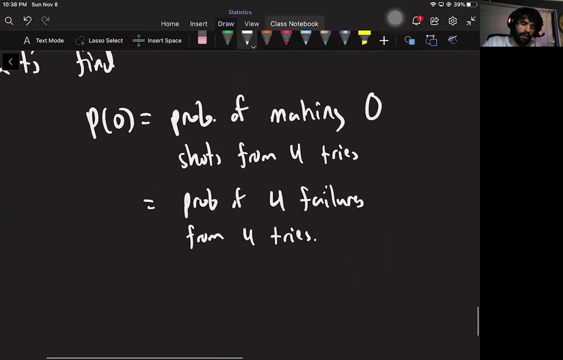 to write it in words, It's the probability Of of making zero shots on four tries, But you can also think about this as probability of four failures from four tries, And what we're going to do is we're going to think about it. 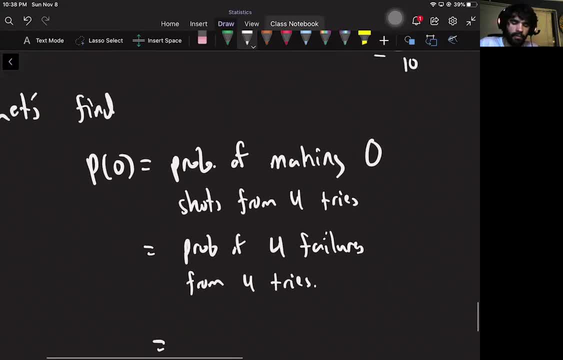 We're going to think about it. We're going to think about it Because they're independent events. We're allowed to multiply probabilities. Each time I throw the basketball, there's a probability that I've, that I make it or that I fail. 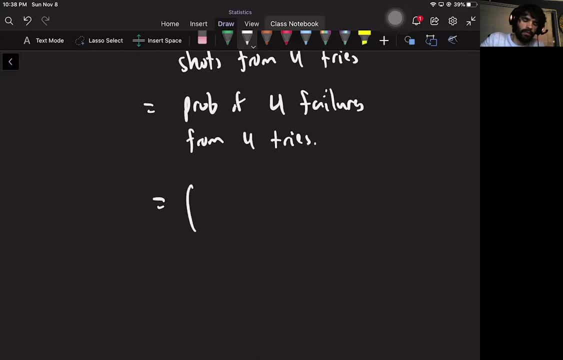 So let's just think about throwing it once. So if I throw it once, what's the probability of missing? What's the probability of failure? Three tenths. So this three tenths represents that I missed the first shot. But now 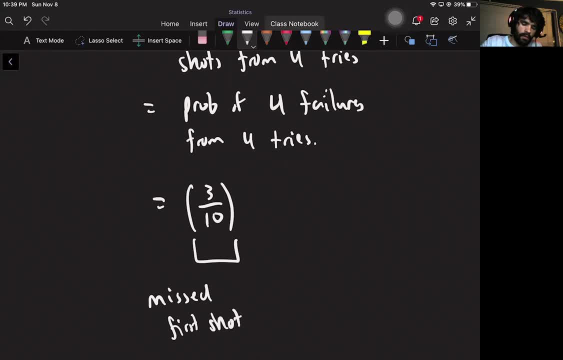 Okay, Okay, Okay, All right, Then let's think about it as five. So let's think about this attorney, and let's think about how amazing. so approximately why, what? how do you use this Among you? how many shots did you miss? 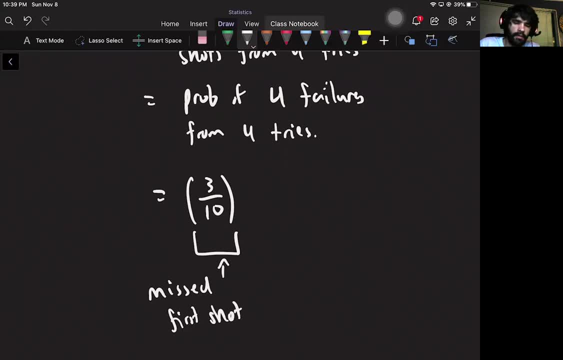 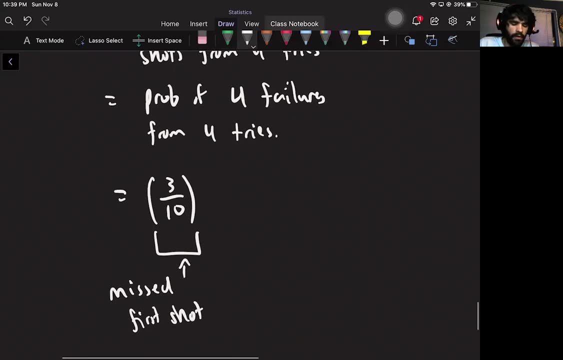 I mean one wasn't a, you know a four or five. did you use a five before? Did you use the five over? and then you're against the rules. I mean, if you're using all your counts in the first order you set, you've gotta see. 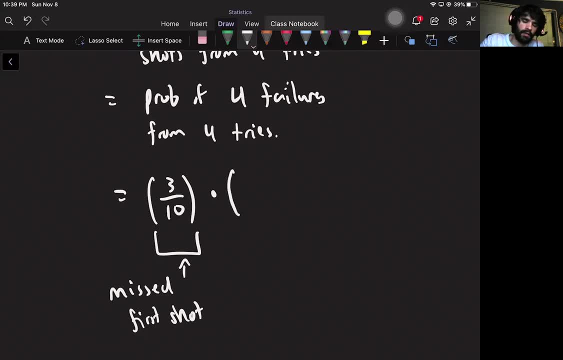 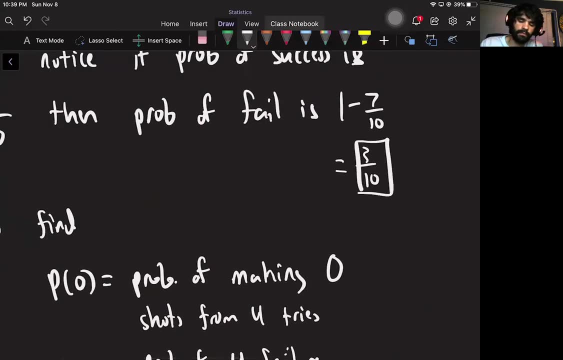 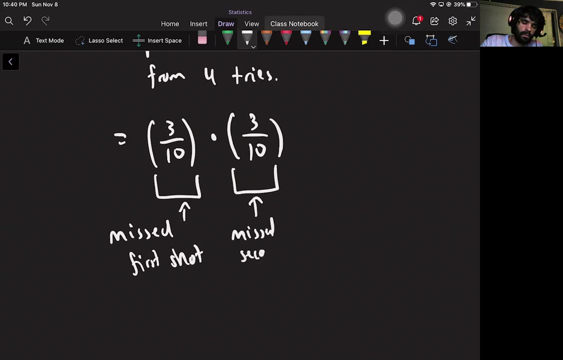 missing the first shot times the probability of missing the second shot, but that's still three tenths. they're all missing is three tenths. that's the probability, probability of failure in this problem. so this is saying that i missed the second shot. because they're independent of each other, i'm allowed to multiply. 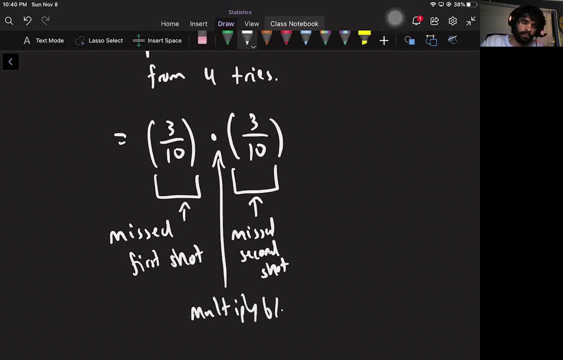 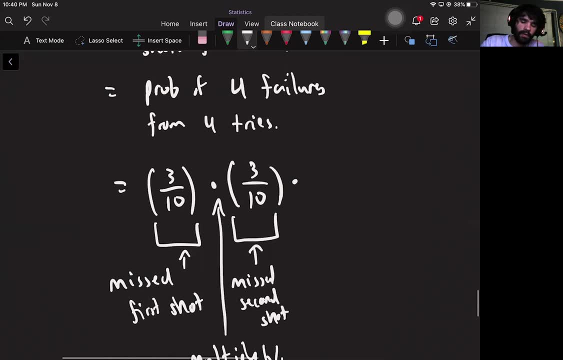 but then this pattern is just going to continue. so now the third shot that i take. i also have a three out of ten chance of failing. so it's the third shot missing. and again i can multiply because it's independent and the probability of doing one thing, and then 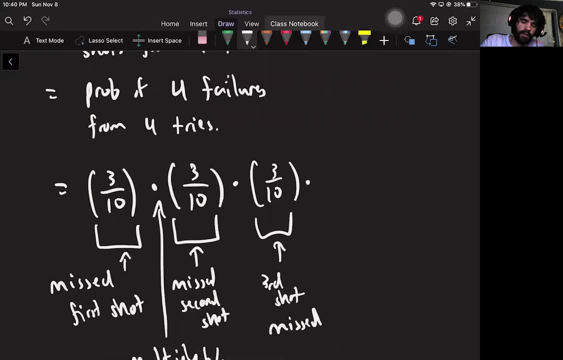 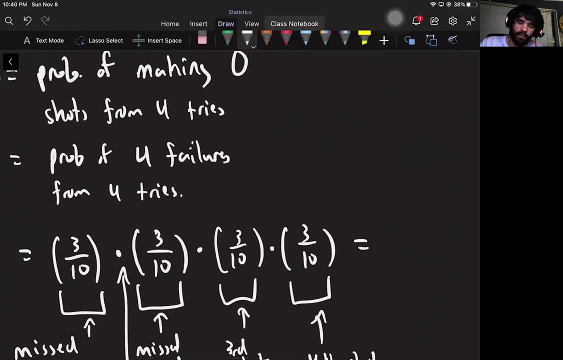 another thing and another thing. let's just figure it out by multiplying them together, and the fourth shot is just one one one. so this is the end. this is the probability of missing all four, and so i can write it like this if i want, but it's fine if you don't. i prefer left out, left separated, so you can see where all the pieces. 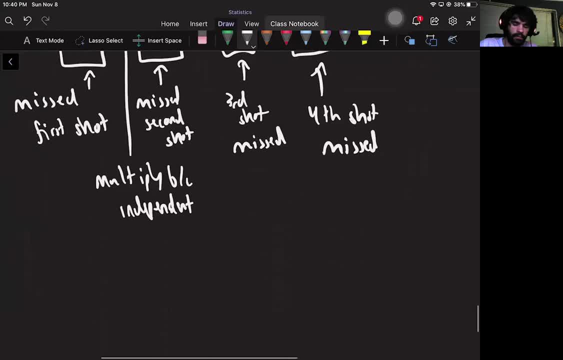 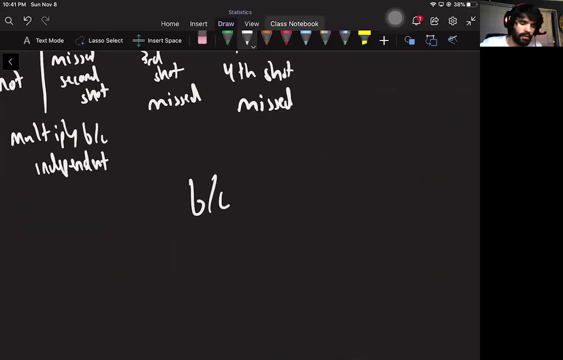 are coming from, um, right? so let me just one more time explain. so this is really because the reason we can do this is because each throw is independent, right? so let me just one more time explain. so this is really because it's really because each throw is independent. 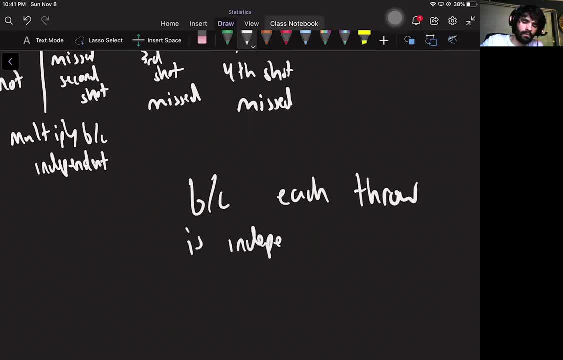 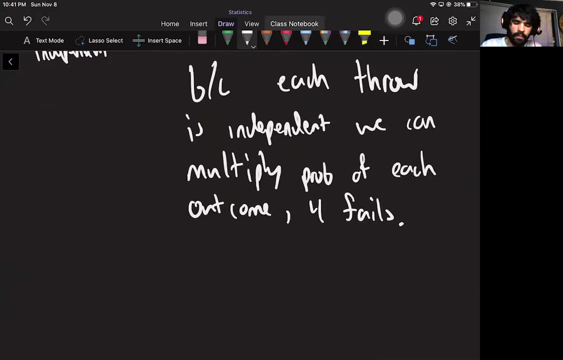 right, so let me just one more time explain. so this is really because each throw is independent of the previous one, so we can multiply probabilities of each outcome, and in this case each outcome is four fails um. so then we can. what else we can do- and this will help later- um is we can. 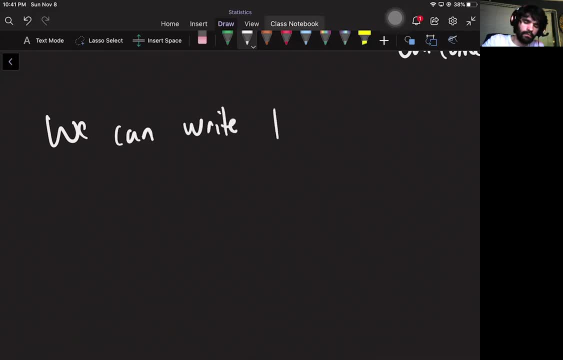 um. so then we can. what else we can do- and this will help later um is we can sort of write out what it means to fail four times using the letter f and writing something like this: so this will come in handy, and what this is saying is that: 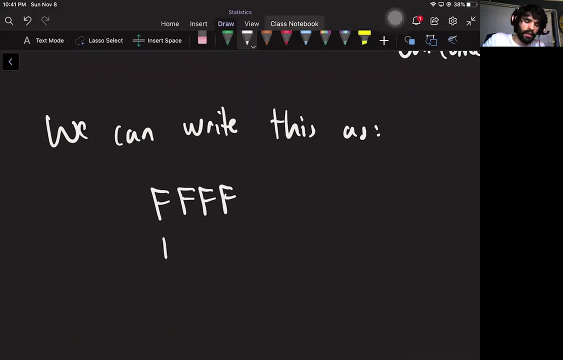 um, this is saying that, like you've, you've failed the first one and the second one and the third one and the fourth one, as opposed to something like we'll see in a second or if i succeed, i'll put an s. okay, um, so that'll come in handy later. it's not so you still get until you see the other ones. 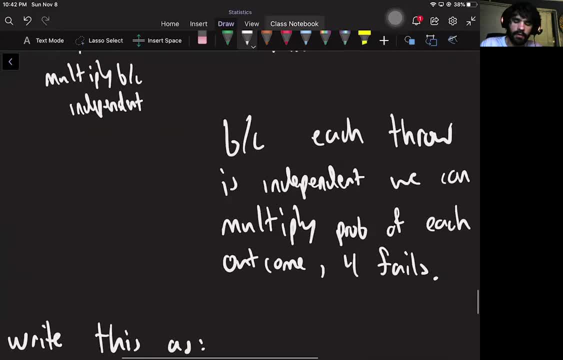 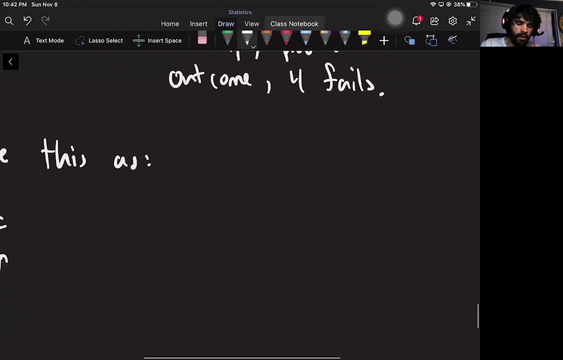 all right, so. so in any case, this is the probability of zero successes right here. that's going to go first in our little chart. once we fill out that chart, what comes after zero one? so now let's figure out the probability of making one shot making- but of course it's one shot out of four tries, because that was established at. 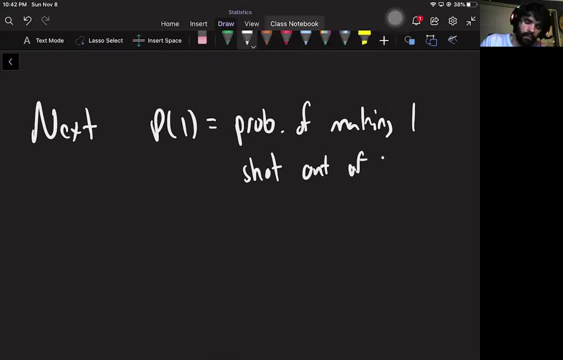 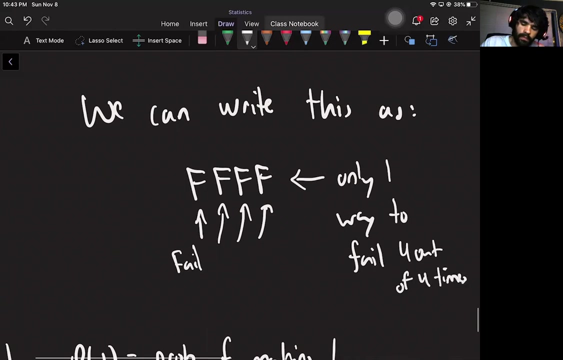 the beginning. you have to establish the number of trials at the beginning, okay, um. so then this one is a bit trickier, because what i would like you to notice is that there's only one way to fail four times. four out of four times, and that's you just do it. you just fail, fail, fail, fail, four times in a row. 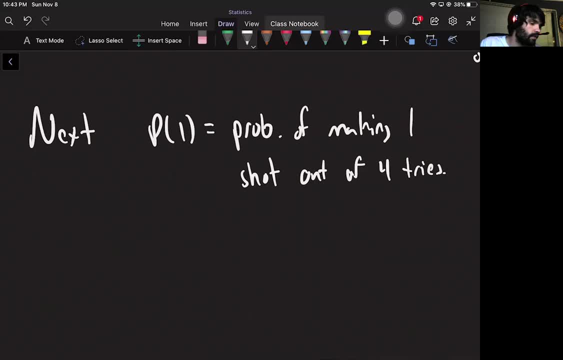 but there's many ways i could fail once. that's the difference, um, and so that's going to affect their answers. so this can happen four different ways. so this is where writing these f's and s's are going to come in handy, um, so what i could do is i could make the first one. 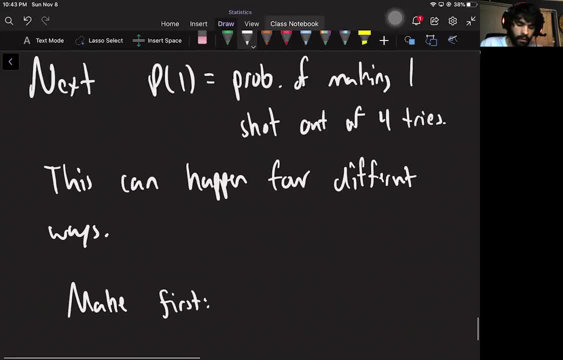 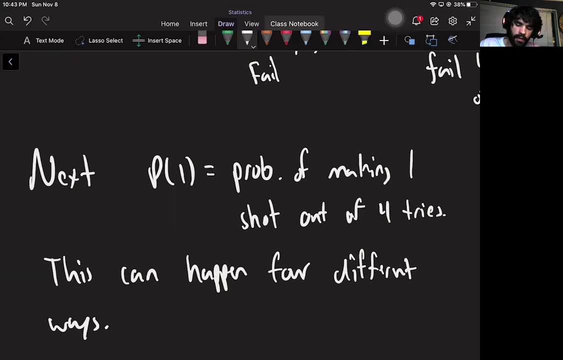 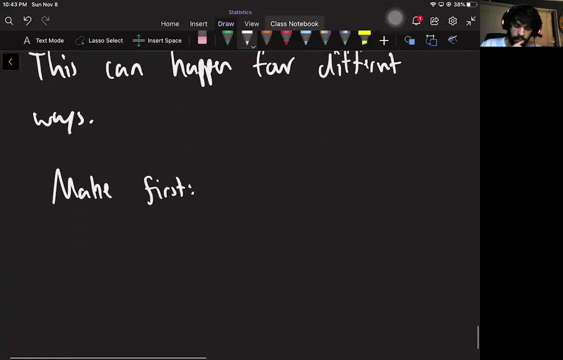 sorry, sorry, yeah, so i could fit, i could. i wrote the right thing. hopefully. i said the right thing earlier, but let me just repeat myself because i didn't. so there's many different ways to fail once, sorry, to fail three times and make it once. that's what i was saying, wrong, so i could make the first one, which i'll write as an s. 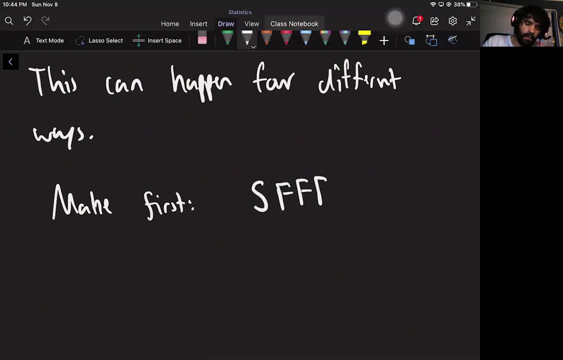 and then i could make the second one, which i'll write as an s, and then i could make the third one, so, and then i could miss the next three. so this is the. this is one way. so this is the. this is one way, so this is the. this is one way to succeed once and fail three times. 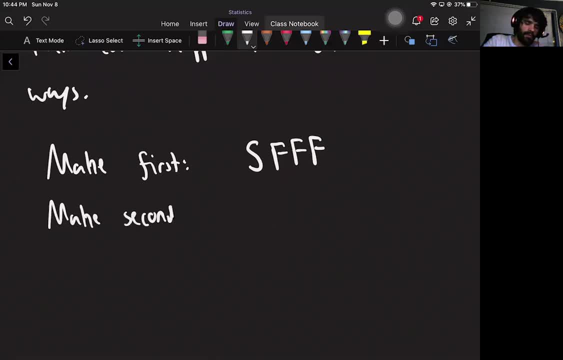 to succeed once and fail three times. to succeed once and fail three times, but but but i could also. instead, i could make the. i could also. instead, i could make the. i could also. instead, i could make the second shot, which i'll write as fs- f, so it's the same that. 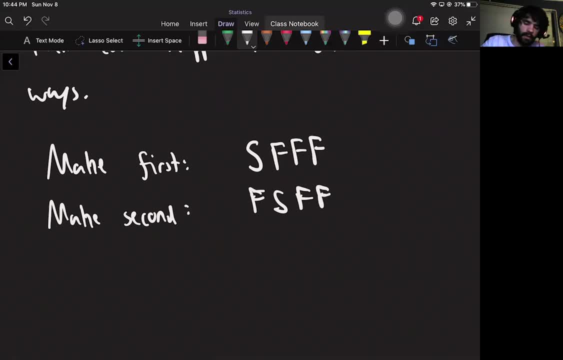 which i'll write as fs f, so it's the same that which i'll write as fs f, so it's the same that i missed the first one, i made the second. i missed the first one, i made the second. i missed the first one, i made the second and i missed the next ones. 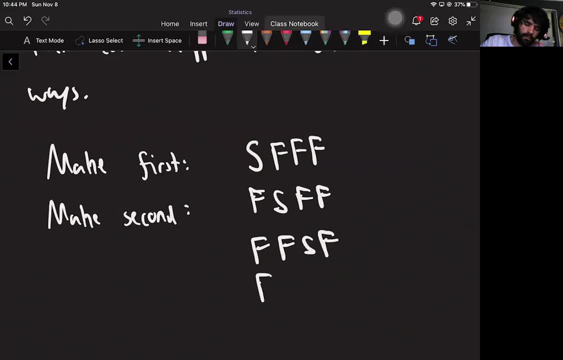 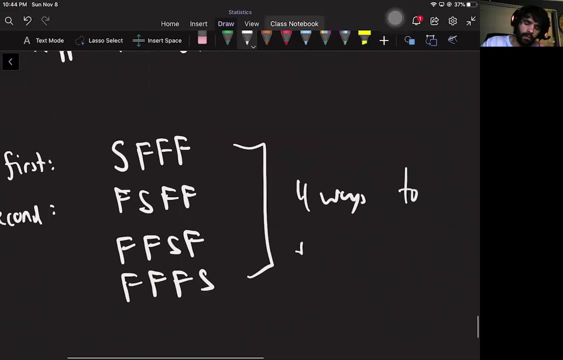 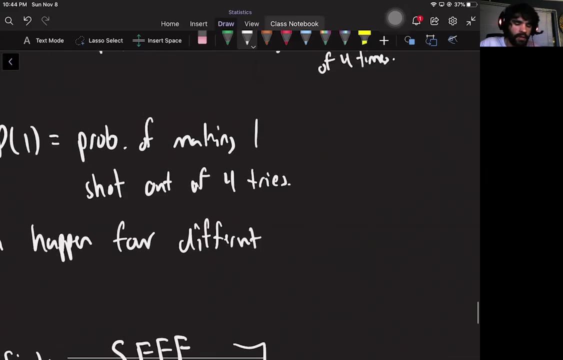 and i missed the next ones, and i missed the next ones, and now we can sort of see the pattern. and so these are the four different, and so these are the four different, and so these are the four different ways to make one shot out of four. so if i'm asking, what's the 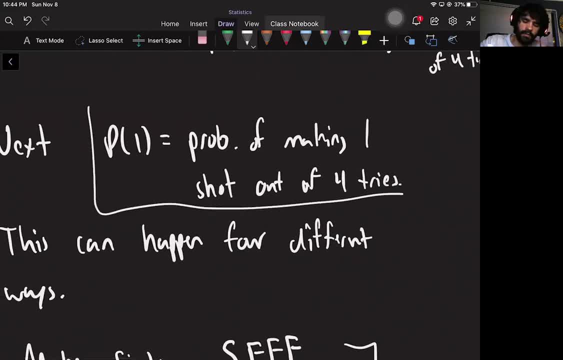 out of four. so if i'm asking what's the out of four? so if i'm asking what's the probability of making one shot out of probability of making one shot out of probability of making one shot out of four tries, four tries, four tries. well, i can do it this way. 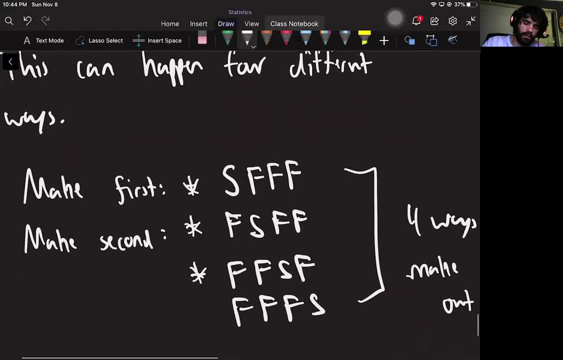 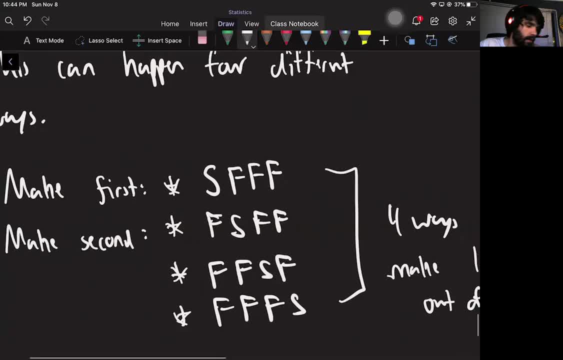 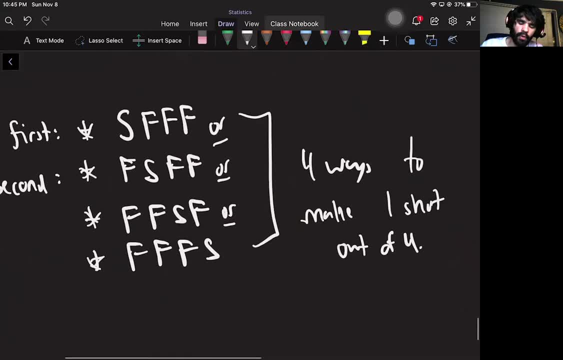 do it this way, or i could do it this way, and the keyword here is or and the keyword here is or, and the keyword here is or um this or this or this or this has um, this or this or this. has to happen, to happen, to happen, and these four ways are disjoint. 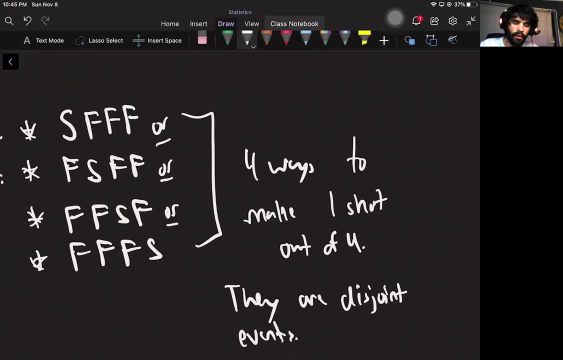 these are all disjoint events, meaning if i. these are all disjoint events meaning if i. these are all disjoint events meaning if i throw four, throw four, throw four free throws. only one of these four can free throws, only one of these four can free throws. only one of these four can happen at that time. i can't do both at. 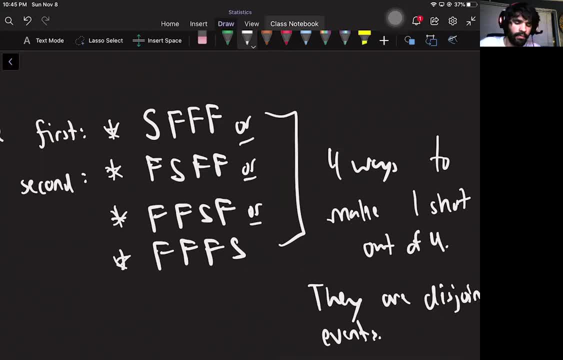 happen at that time. i can't do both at happen at that time. i can't do both at the same time because i can't miss the same time, because i can't miss the same time, because i can't miss the first, the first, the first, and miss the second and still have. 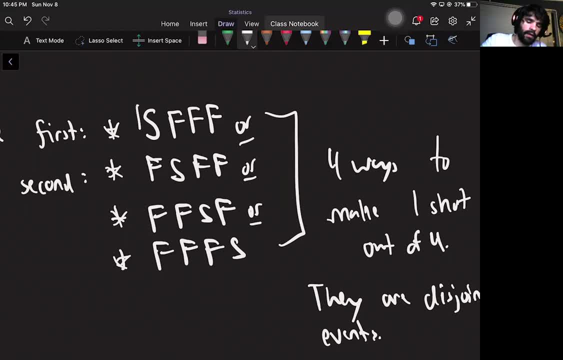 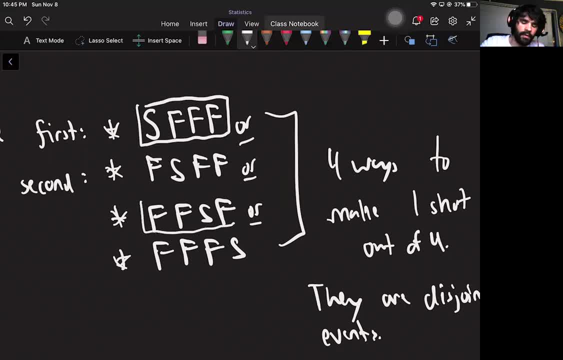 first. first miss three and then, at the same time, miss three and then, at the same time, miss three and then, at the same time, somehow, somehow, somehow make the third one and miss the others. it make the third one and miss the others. it make the third one and miss the others. it just doesn't make sense. 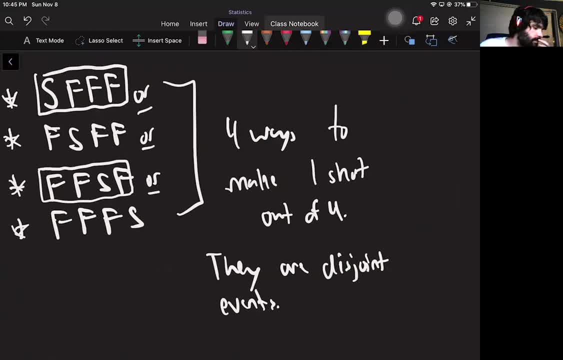 just doesn't make sense. just doesn't make sense. only one of these events can happen at. only one of these events can happen at. only one of these events can happen at a time. so they're disjoint a time, so they're disjoint a time, so they're disjoint um so. 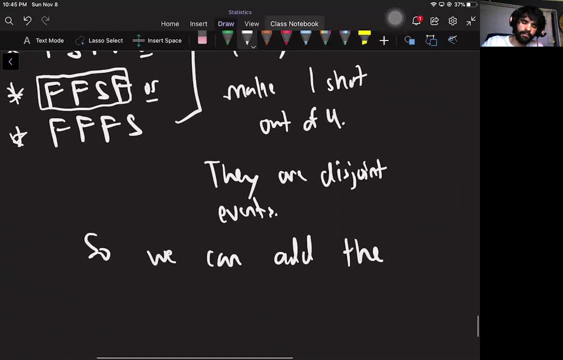 um, so, um. so we can add that the probabilities of, we can add that the probabilities of, we can add that the probabilities of them happening, to figure out the probability of one success, the probability of one success, the probability of one success, because there's only these four ways to. 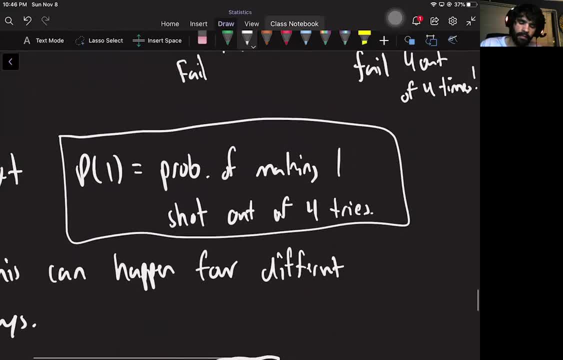 because there's only these four ways to, because there's only these four ways to do it. so if i just figure out these four, do it. so if i just figure out these four, do it, so if i just figure out these four probabilities, i can add them up and 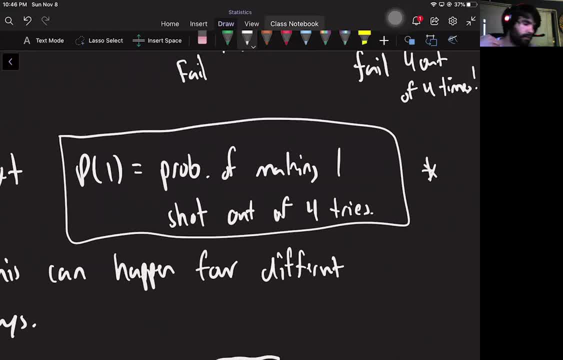 probabilities, i can add them up. and probabilities, i can add them up and that'll tell me the probability of me of that'll tell me the probability of me of that'll tell me the probability of me of one success of making one out of four. one success of making one out of four. 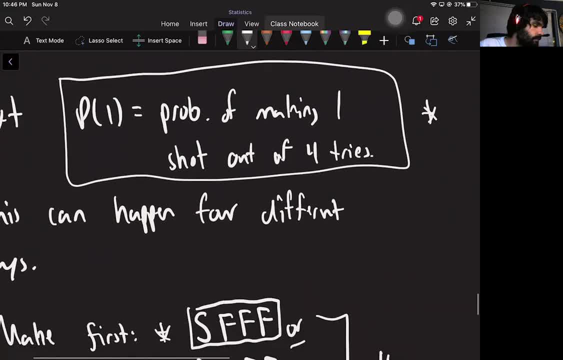 one success of making one out of four trials, trials, trials, um, and this won't be so bad, um, and this won't be so bad, um, and this won't be so bad okay, so let's do it. so what's the okay? so let's do it. so what's the? 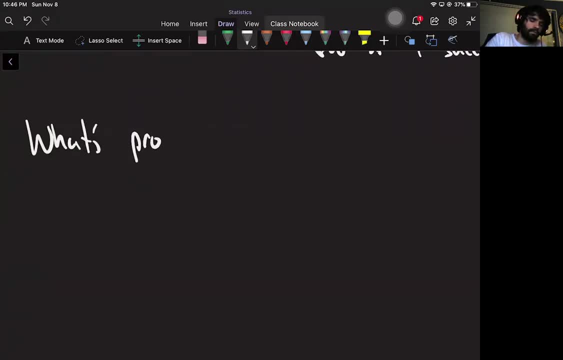 okay, so let's do it. so what's the probability of the first meaning i: i succeed once and then i fail. meaning i: i succeed once and then i fail. meaning i: i succeed once and then i fail three times after that, three times after that, three times after that? well, i'm just going to do what i did. 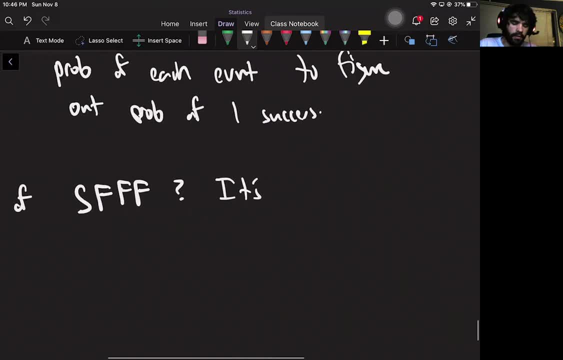 well, i'm just going to do what i did. well, i'm just going to do what i did before, before, before. because these four events are, because these four events are, because these four events are independent. i succeed, then i fail, then i independent. i succeed, then i fail, then i. 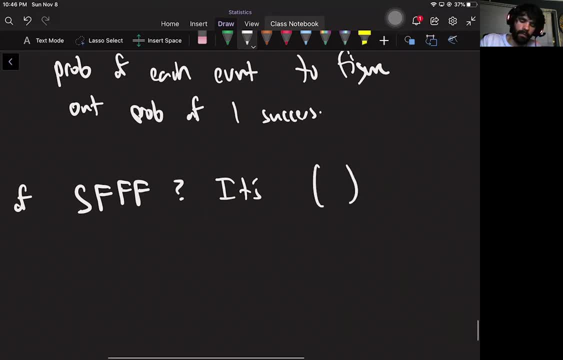 independent. i succeed, then i fail, then i fail, then i fail. fail, then i fail, then i fail, fail, then i fail, then i fail. i can just multiply the probabilities of each event, the probabilities of each event, the probabilities of each event happening. so what's the probability of? 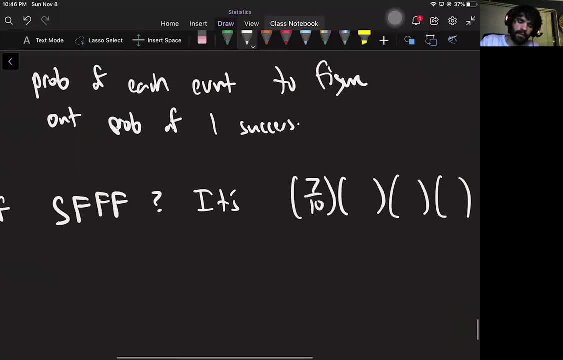 happening. so what's the probability of happening? so what's the probability of success? from the beginning of this success, from the beginning of this success, from the beginning of this problem, it was seven out of ten problem. it was seven out of ten problem. it was seven out of ten. so this is saying that i make the first. 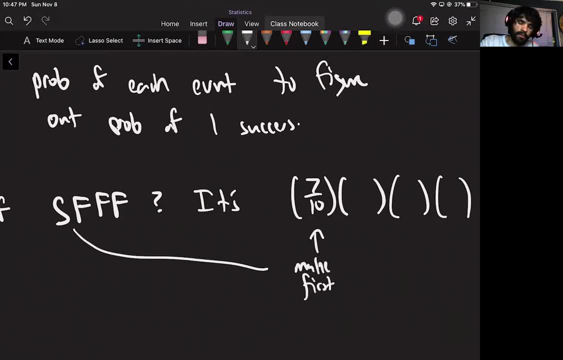 so this is saying that i make the first. so this is saying that i make the first, just like that's what that s was standing for um. that's what that s was standing for um. that's what that s was standing for um. and then what was the probability of? 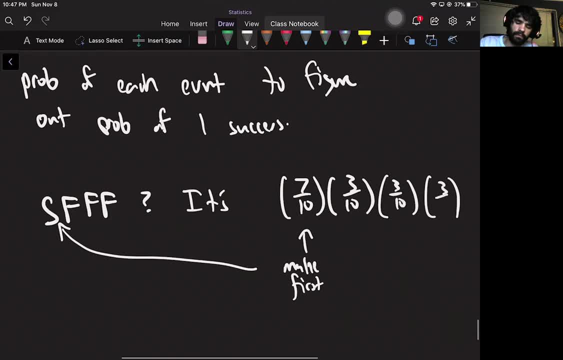 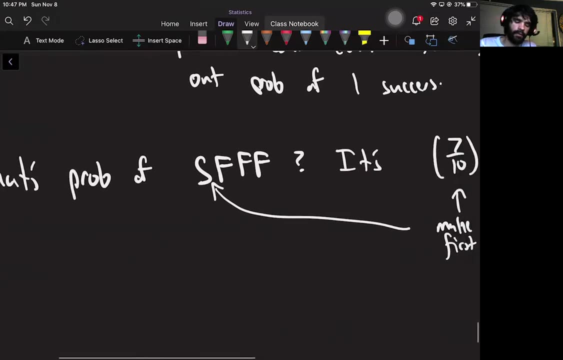 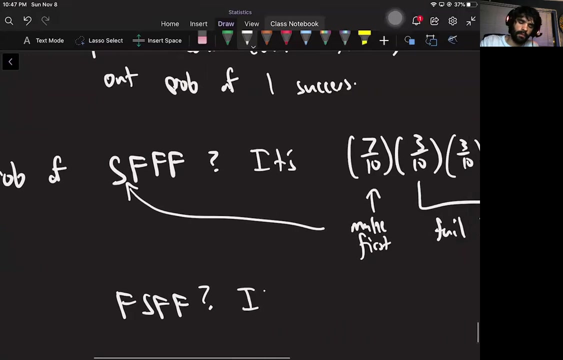 and then what was the probability of? and then what was the probability of failure? that was three out of ten. so those are then fail: three um now, um now, um now. So that's the probability of that happening. What about of this one happening instead? Same idea. 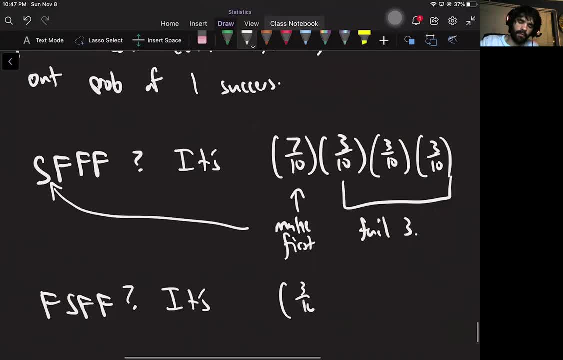 Well, now I've failed the first one, so that's gonna be three out of 10.. I make the second one, so that's gonna be seven out of 10.. Then I fail, then I fail again. So now we can see the pattern. 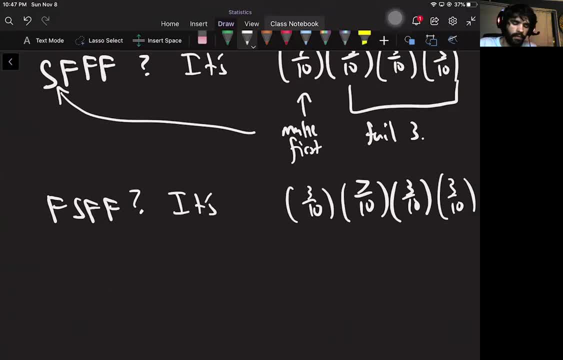 Wherever there's an S, I'm just putting the probability of success. Wherever there's an F, I'm putting the probability of failure. So the next one and the next one. after that. I can get very easily by just doing the same pattern. 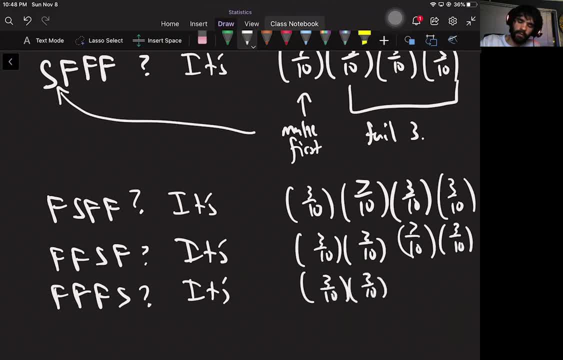 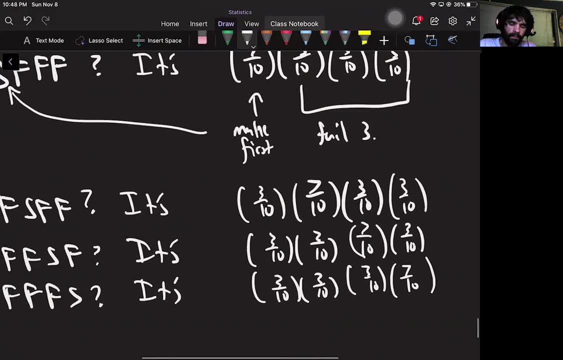 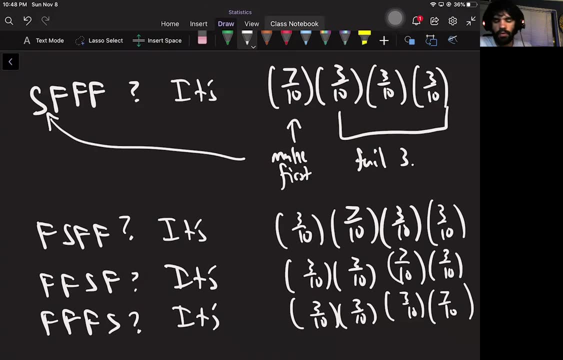 So the last one is gonna be fail, fail, fail and then finally succeed on the last try. So these four probabilities correspond to the probabilities of these four different disjoint events happening, of either making the first one or instead making the second one, or instead making the third or making the fourth. 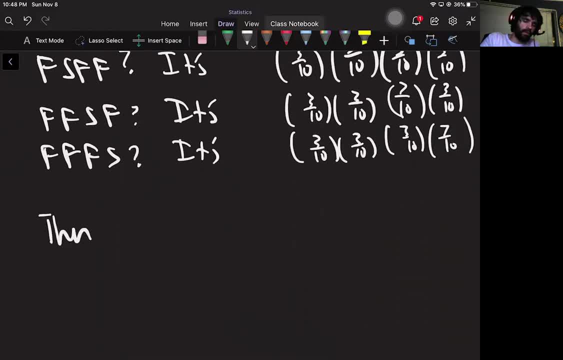 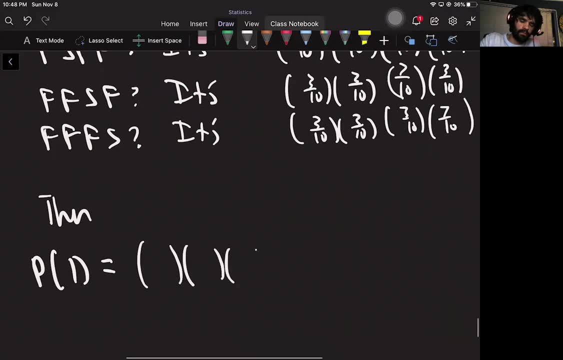 So then, finally, I just have to add all these up, And that's the probability of one success out of four tries. It's gonna be this giant thing, So I could make the first one and then miss the next ones, Or I could, and that's why I'm adding. 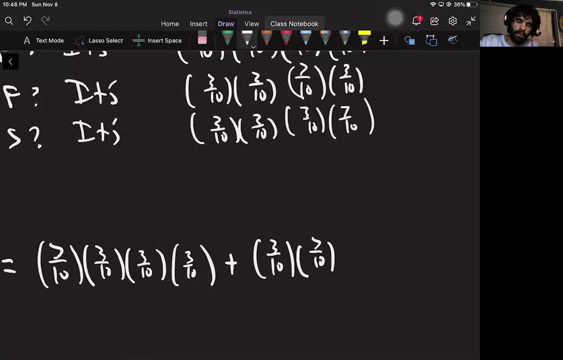 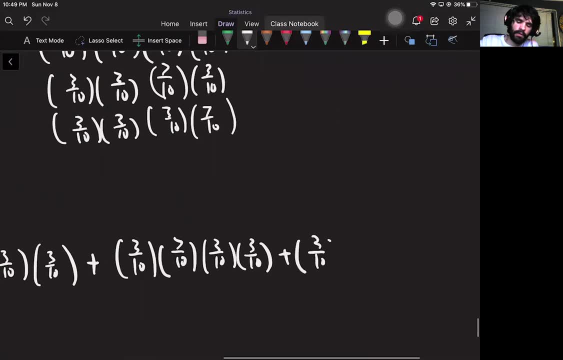 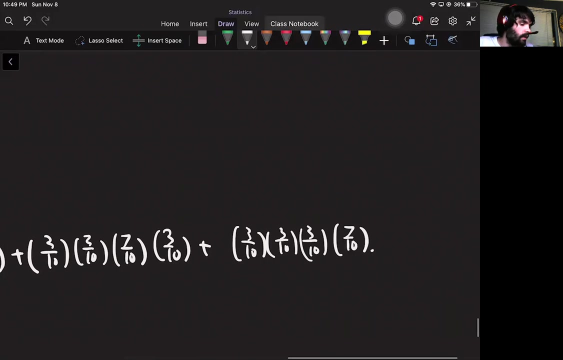 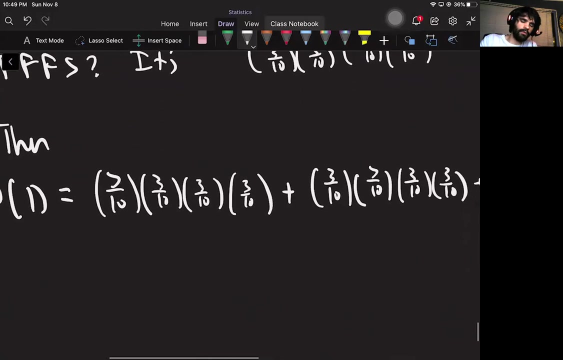 I could miss the first, make the second, miss, miss, or I could miss, miss, make it miss again, and then, finally, I could miss the first three and then make the last one. But if you know some math, these four numbers are the same number because all they are the same, four things being multiplied together in different orders. 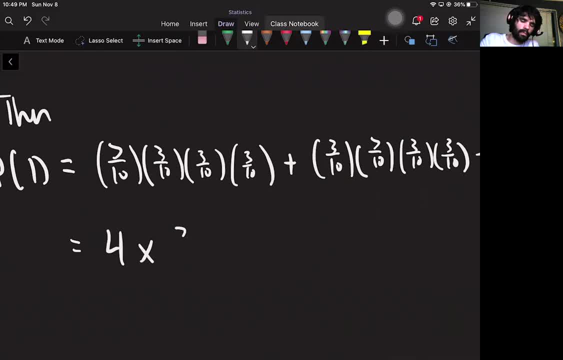 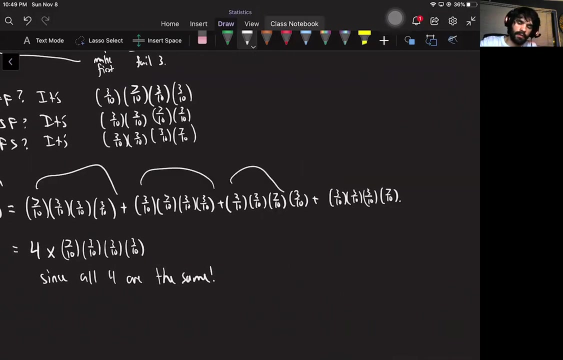 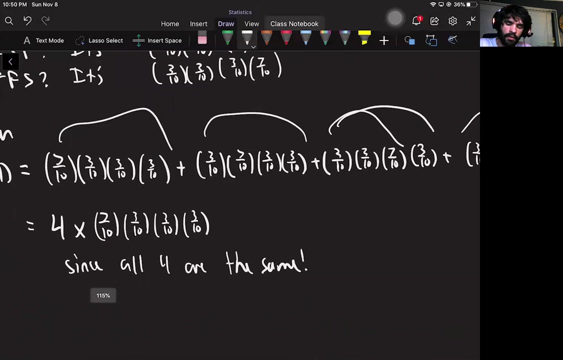 So this is really four times the same number. So that's the shortcut. If I add for the same thing, I can just multiply by four. right, so just zooming out here: This, this, this and this are all the same number, because they are the same numbers multiplied together in different orders. 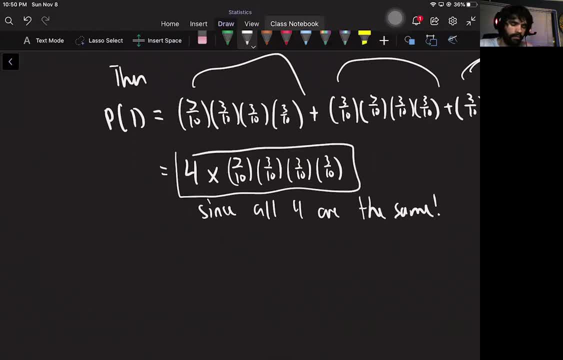 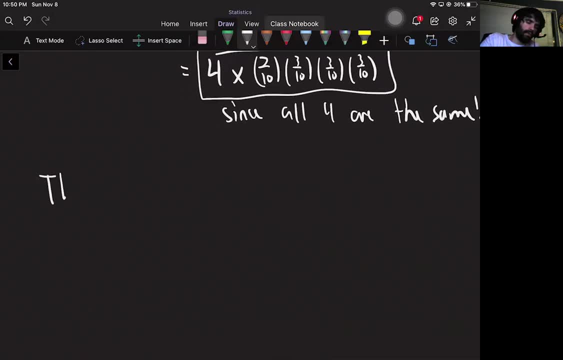 Okay, so then this is really the probability of one success. So now we can sort of speed up a bit. So what about probability of to accept to success? So I'm making two out of four tries. Well, the quick way to do it now is list out all the ways to do to make two out of four tries. 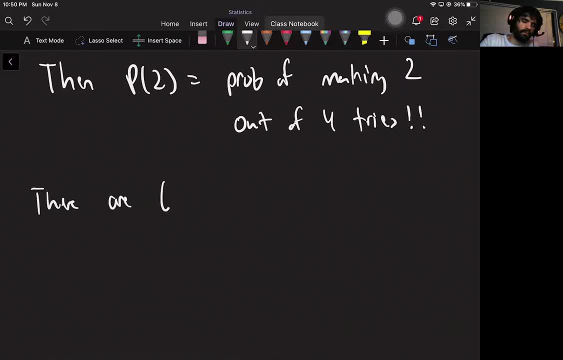 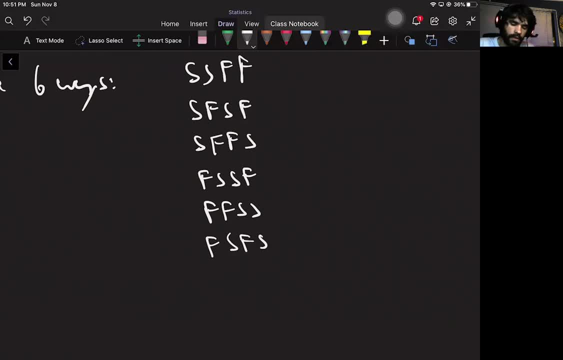 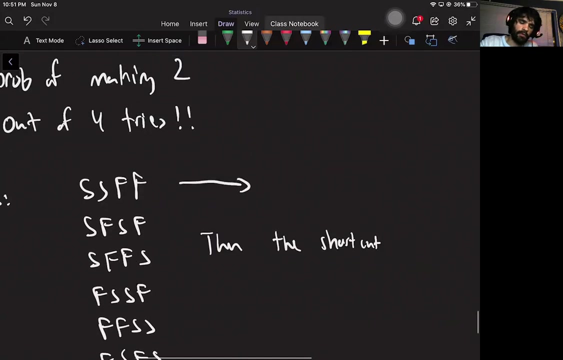 Now succeed, fail, succeed, and that's six, overall six. So what this means is the shortcut, The probability of this first guy happening, of making the first two and then missing the next two, is just the probability of making it times. the probability of making it times the probability of missing has a probability of missing. 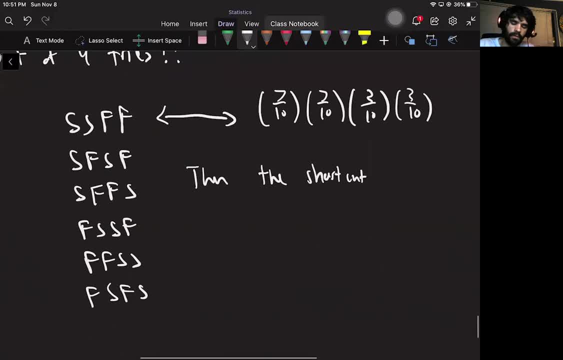 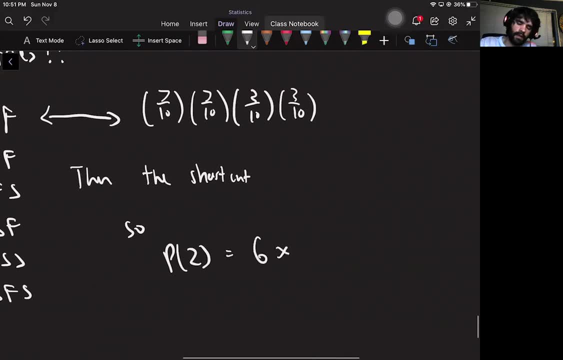 But then all six of these are the same, So the probability of two successes is just six times that number. So there's six different ways. I could succeed twice and fail twice out of four tries. So then, but really it comes from adding on all six things. 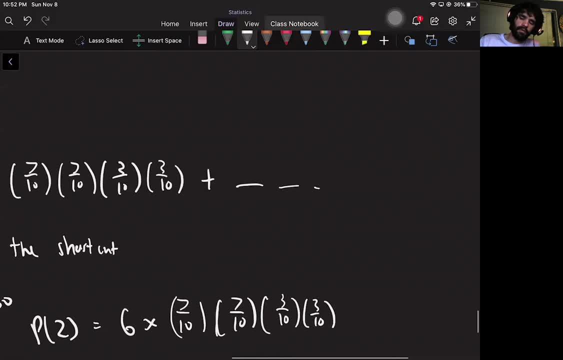 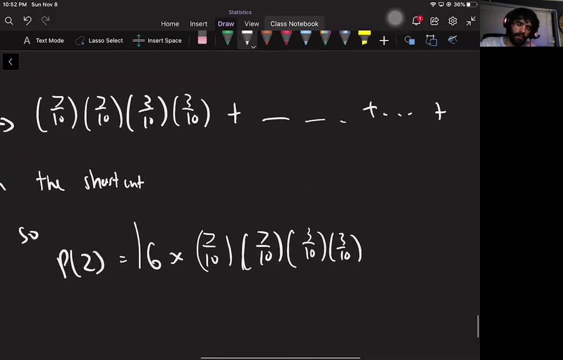 So you're really adding this plus the next one, plus the next one, which I we did before, but there's six of them and they're all the same, So I'm not going to do that. Instead, I'm just going to multiply the first one by six, because they already know they're the same. 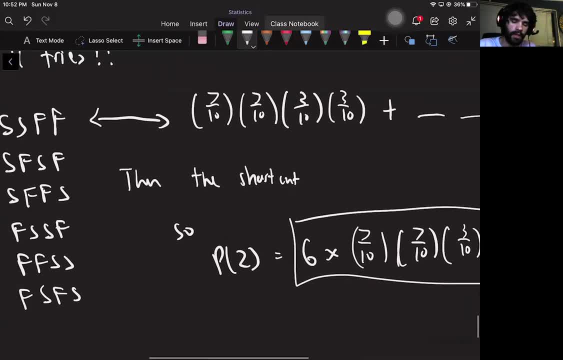 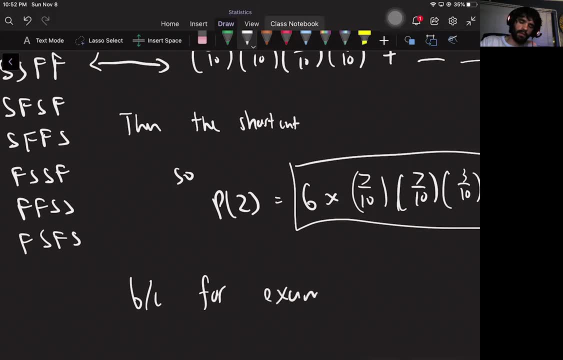 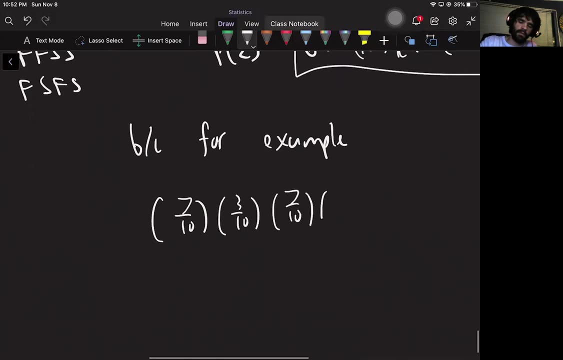 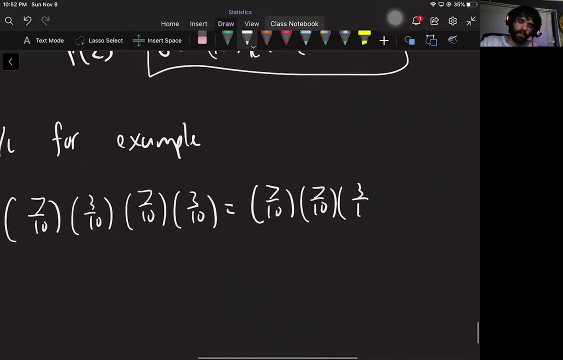 Just because when you switch the order of multiplication it doesn't change the number. So just for a mini example of what's going on: Seven over 10 times three over 10 times seven over 10 times three over 10, that's exactly the same as if I just do a 710 to the front. 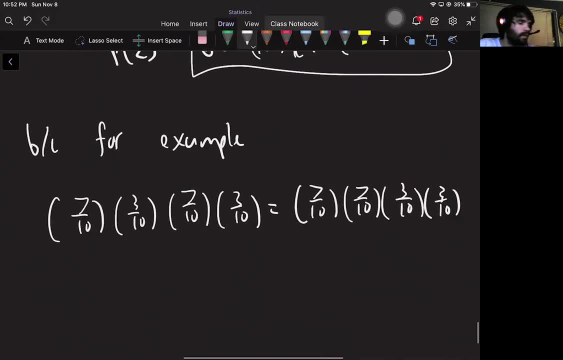 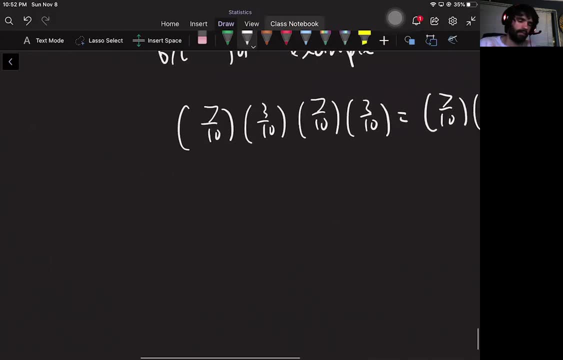 The order of multiplication. You can switch around there. Multiplication, Okay, So that's why you can just multiply by six. So then next is three. Well, I can sort of start skipping ahead that this. this just means I want three successes. 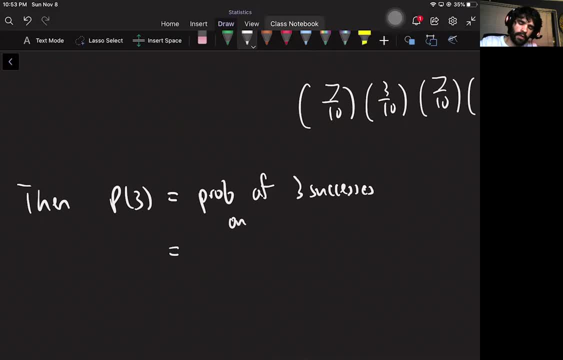 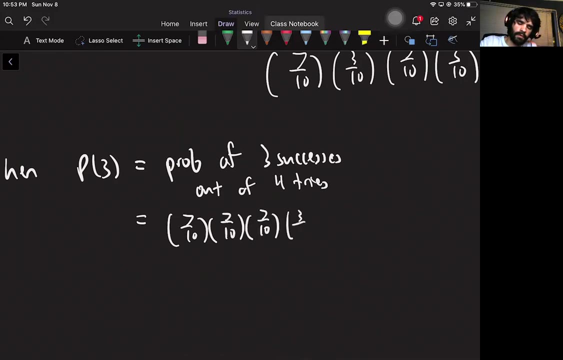 And out of four tries, And now I sort of see the pattern. It's just: every time I get a success, I do the probability of success. I'm going to have three of these and one of fails, But then how many ways are there to do this? 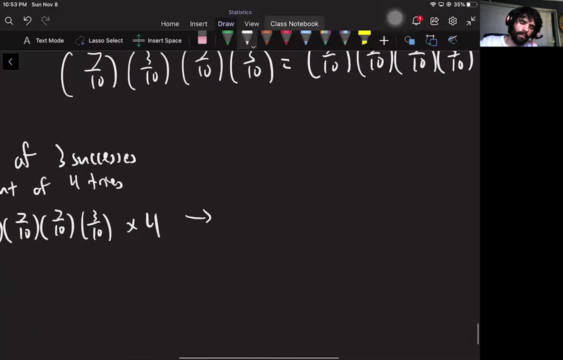 There's going to turn out to be four different ways. There's four ways to succeed three times. So you can write about if you want, But they just sort of are the opposite of failing three times. Just sort of two sides of the same coin. 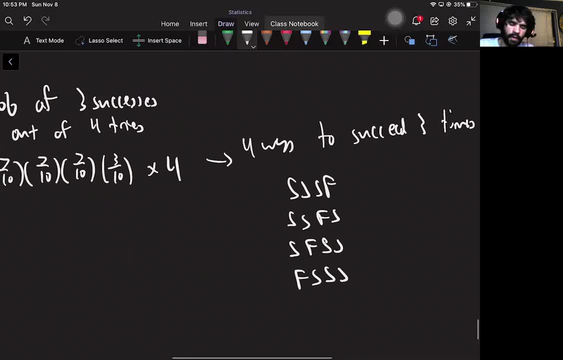 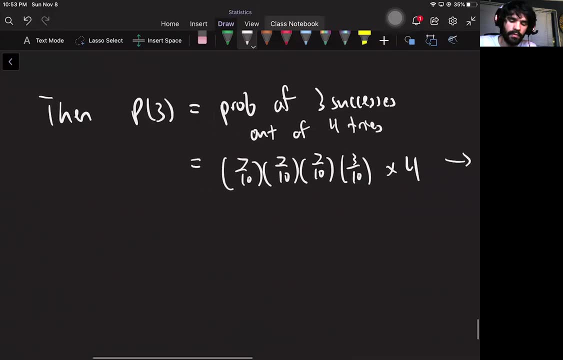 Succeeding three times versus failing three times are just sort of the opposite. And there was four of the failing three times, Just like there's four of the succeeding three times, And then, lastly, P of four. Well, there's only one way to succeed. 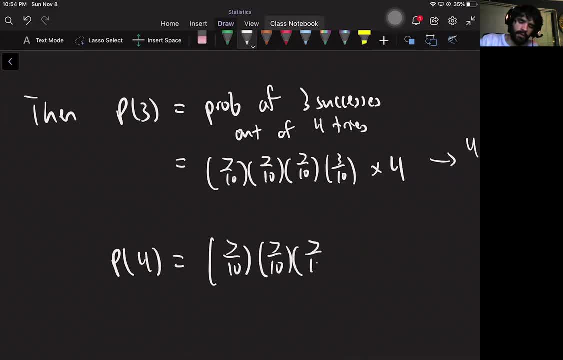 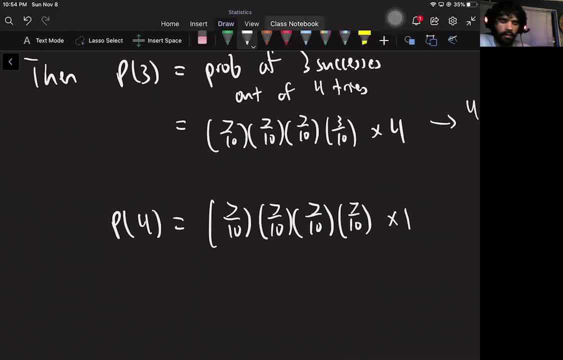 Four times out of four times, And let's just do it. You just succeed every time. There's no other way to do it. So if you want, you can put a times one, just to have it look symmetrically. There's only one way to succeed: four out of four times. 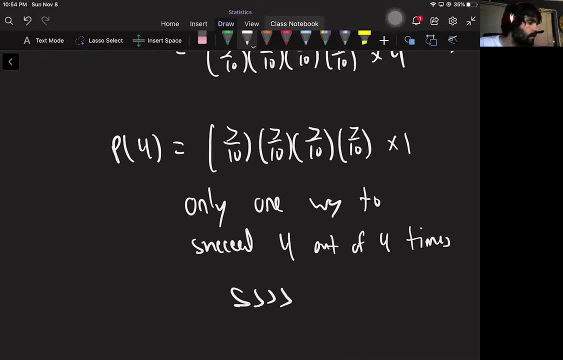 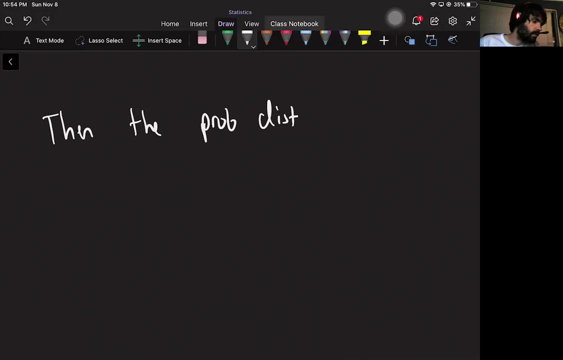 Let's just do it Four S's. Okay. so then this finishes the problem. So now we could write out the probability distribution For this binomial experiment, So I guess I could call it the binomial probability distribution. Is So my number of successes that are possible are on the left. 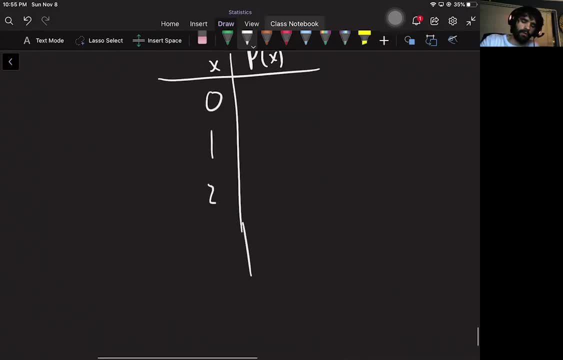 So I can do 0,, 1,, 2,, 3 or 4.. And we figured all these out. So zero was Just a bunch of three out of tens, And you can multiply together if you want. One is just one success. 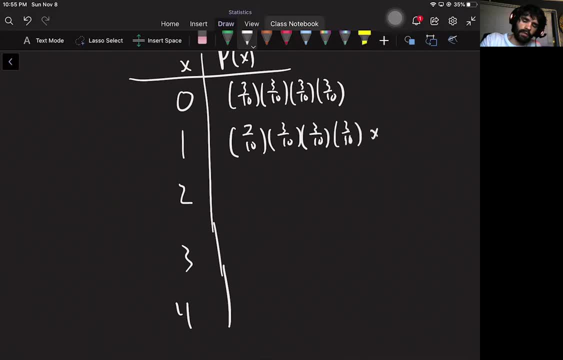 And three fails. But because there were four different ways to do that, I have to multiply by four, And then there's Succeeding twice. Failing twice gets me this: There were six ways to do that. Now I'm succeeding three times. 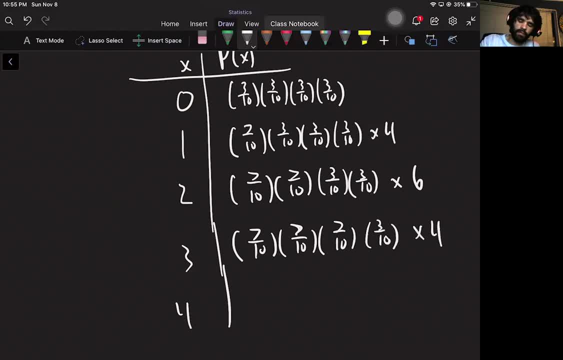 Failing once Four ways to do that And then finally I'm succeeding all four times out of four. Oops, And There's only the one way to do that. So I'm going to write a times one. It doesn't really matter, just to look sort of proportional. 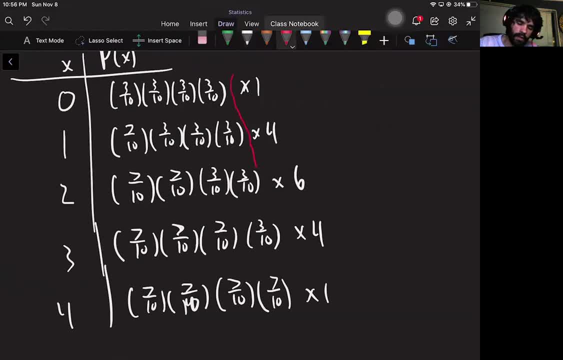 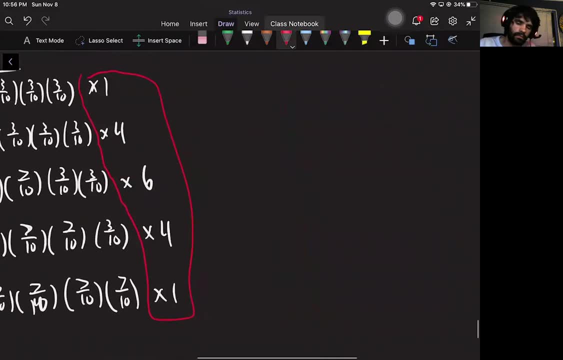 And that's because these numbers are very important and you might Recognize them from something called Pascal's triangle, But if not, that's okay. What I do want you to notice Is that these numbers Have nothing to do with the probability. 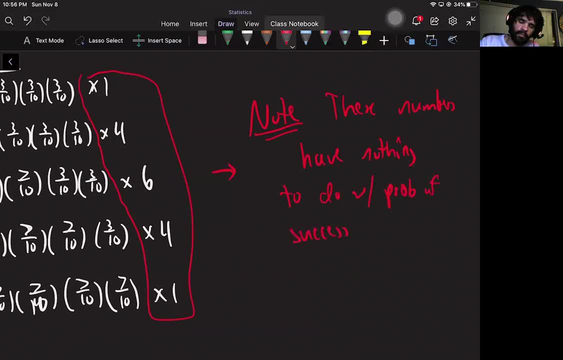 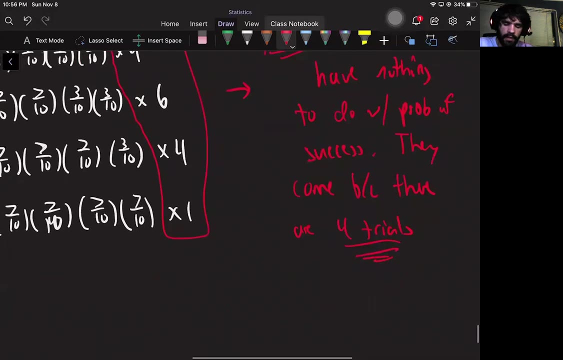 Nothing to do with the probability of success. They came from The number of trials And The probability of success. So what this means is: as long as there's four trials. That's what dictated These numbers, because they came from drawing out these. 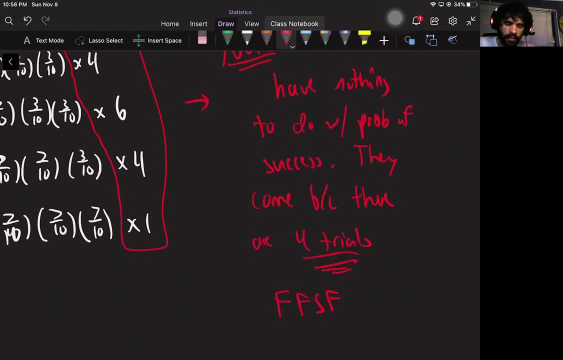 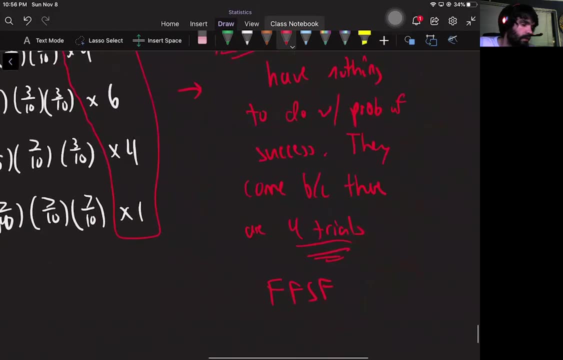 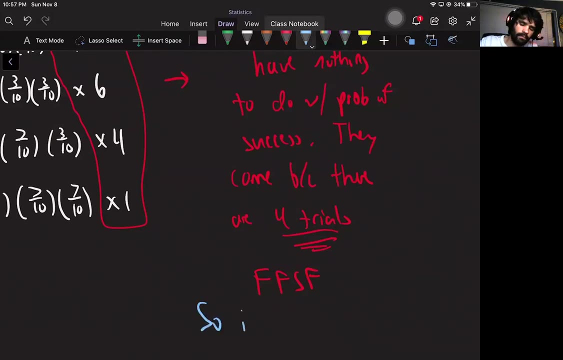 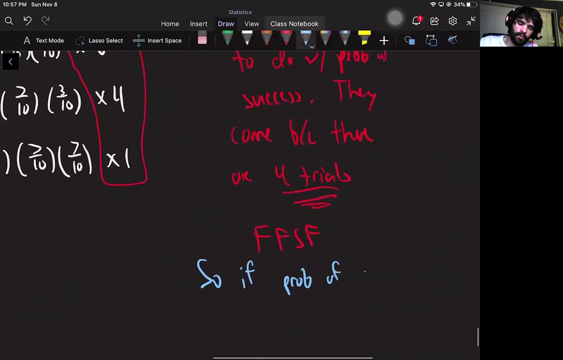 Little things like this. But if there are five trials or six trials or three trials, you would draw A different amount. So what that means is, if I change the probability of success to something else, Then These four numbers, with these 14641, would stay the same. 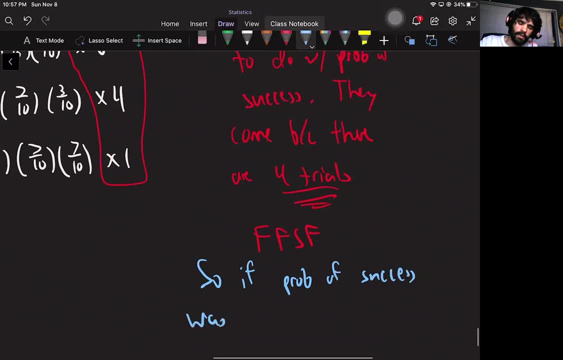 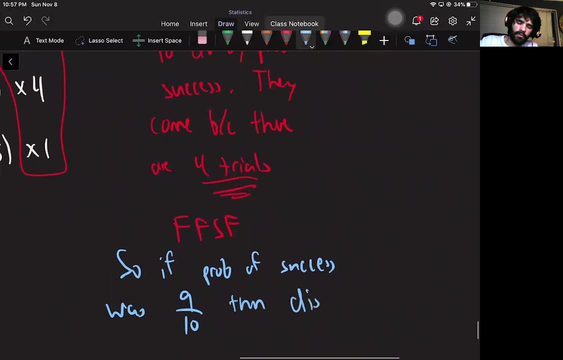 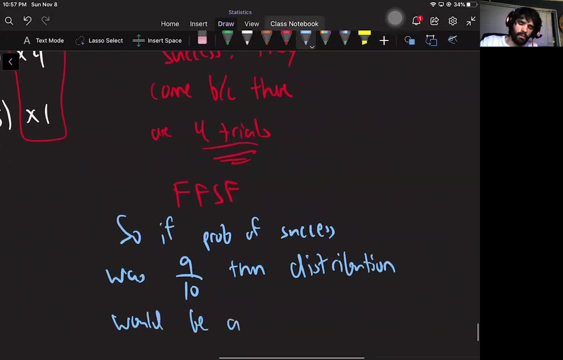 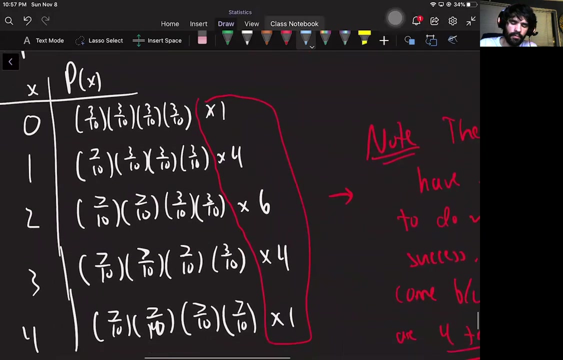 So, for example, if the probability of success Was, say, someone better than me to quickly throws and 10. Then The binomial distribution, You could fix it very easily. It would be almost the same, Because These numbers In red here would stay the same. 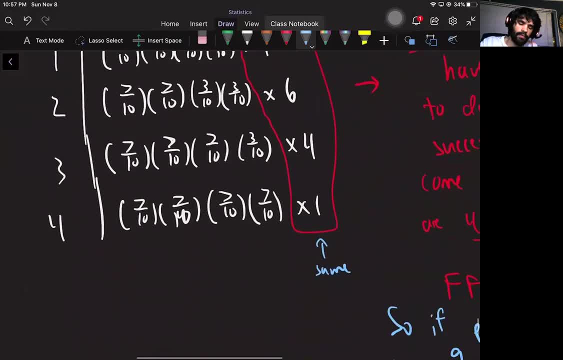 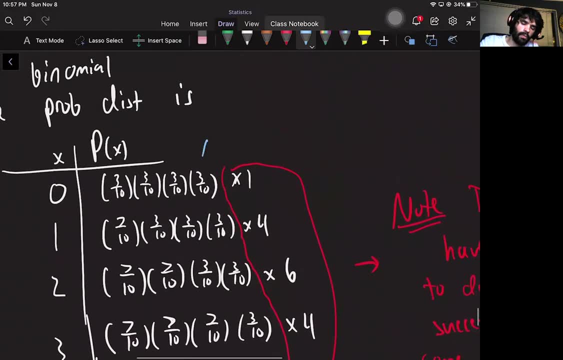 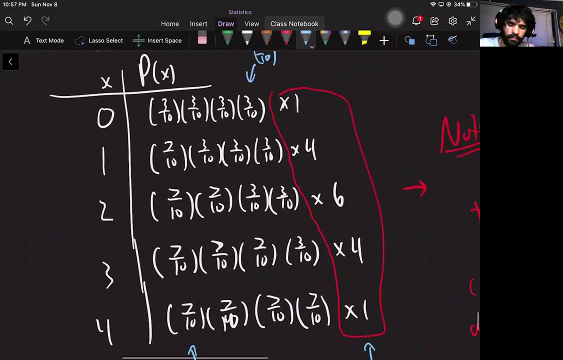 What would you change? You would just change the successes To nine out of tens, And therefore the fails I have to change to One out of tens, And that'd be it. So that's nice. So If I change the number of trials to like five, though, then these will be a. 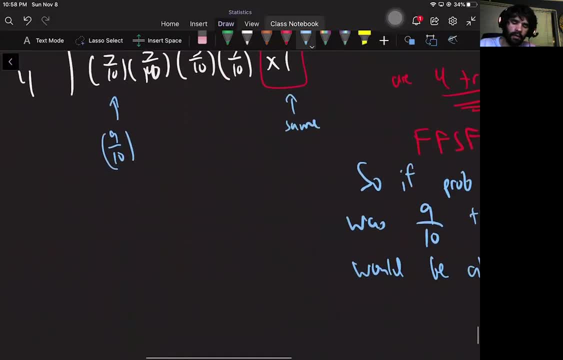 little bit different. You have to figure them out By drawing All the different ways. For example, to succeed Once and fail four times out of five, And then you have to draw the rest to figure out how many there are. Okay. 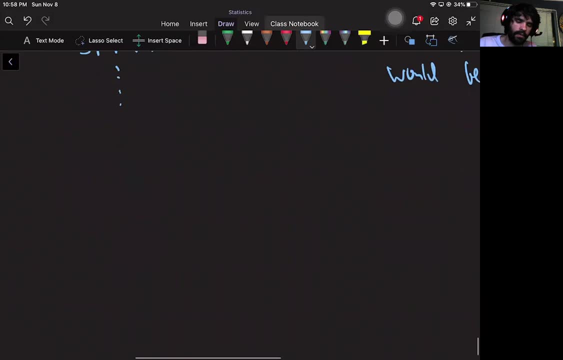 But that's for other examples. So now, the last thing we want to do with these. The reason that they're so nice Is the following: So binomial distributions, Or binomial probability distributions, Have relatively Simple formulas For The mean, AKA the expected value. 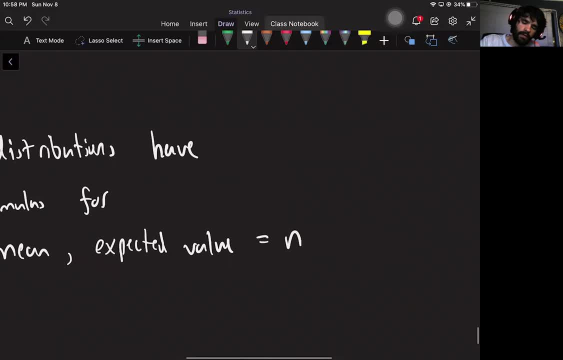 It turns out to just be N times P, or N is the number of trials And P is the probability of success. Okay, So remember how to actually calculate this expected value thing. This bad boy was horrible to calculate. How do you do that? 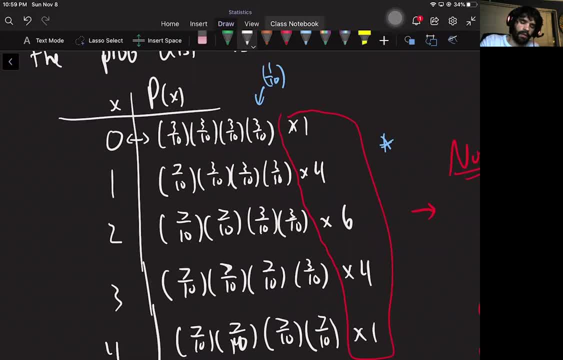 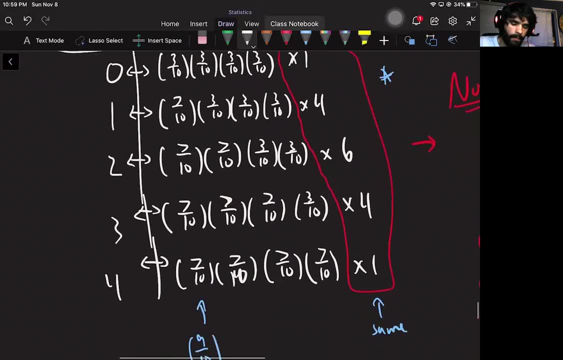 You have to do The X times- it's probability, And then the next one, and then the next one, And then the next one, all of these multiplied to their corresponding probabilities, And then you have to add them all up, Right. 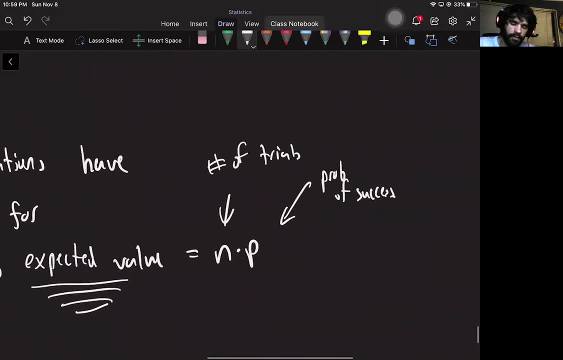 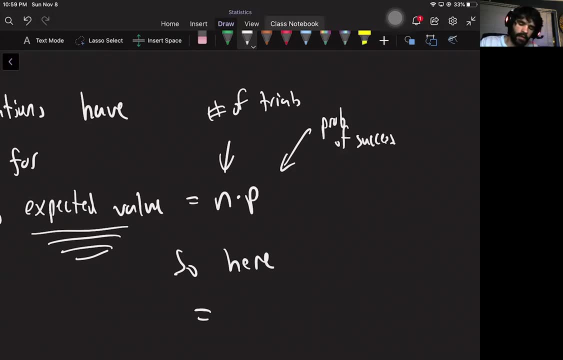 It was terrible. That was the expected value. Well, there's a shortcut: If it's a binomial probability distribution, then you have to calculate the expected value. So here, If you did that long giant process, it would turn out to just be. 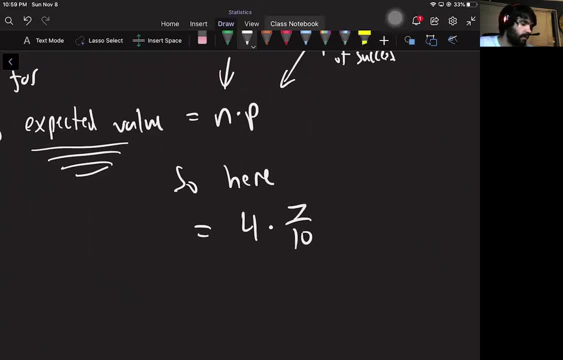 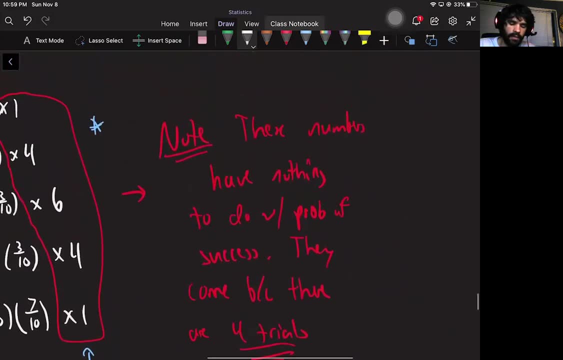 Four times Seven out of 10, because there were four trials in that example, The probability of success would Seven out of 10.. So it would just be that. So you actually did the wrong way to calculate expected value. It would just be horrible. 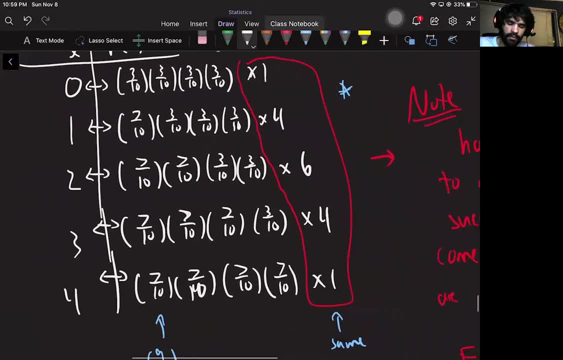 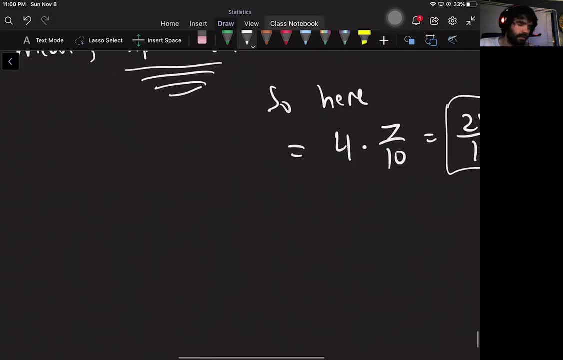 It takes so long, But it would turn out to be the same as just 28 over 10.. You can verify it if you want, or you can believe me, But it's very long. Okay, And the standard deviation was the other type of thing we calculated. 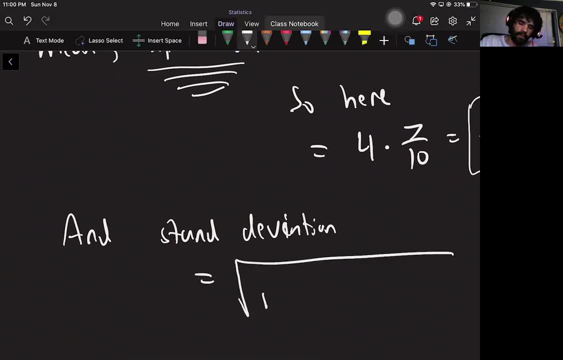 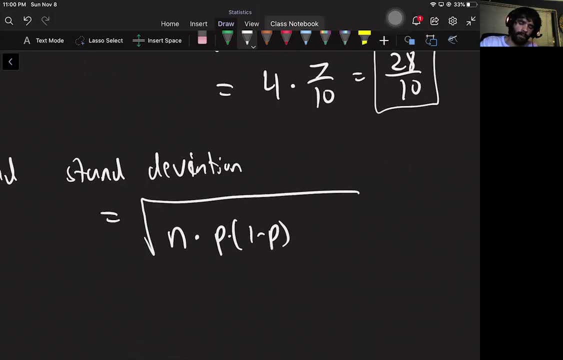 Also has a nice formula. It's just the square root of n Times p times one minus p, AKA the square root of The number of trials And then the probability of success. What's one minus p? then? That would be the probability of failure. 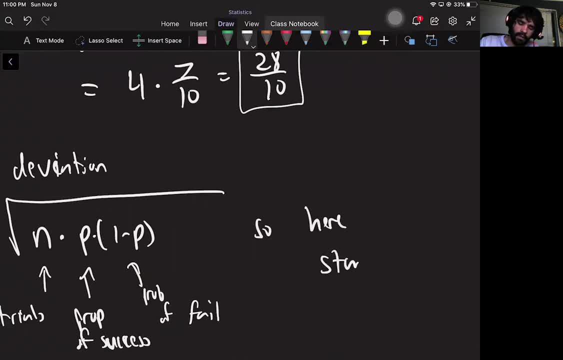 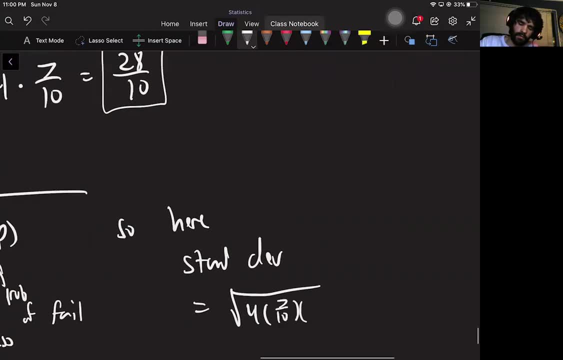 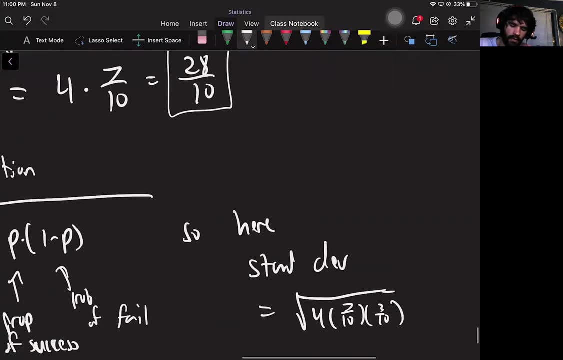 So in this situation The standard deviation is just going to be Square root of four times Seven out of 10 times three. So whatever that is in your calculator, That's the standard deviation. And, as a way, way, way. 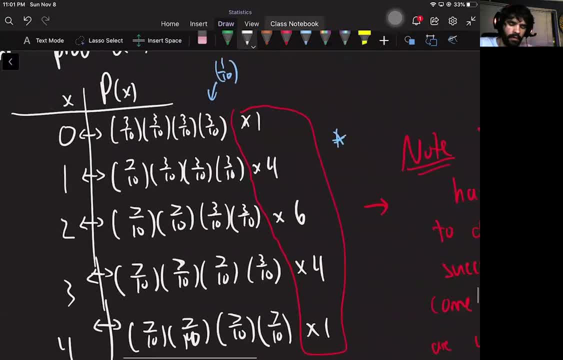 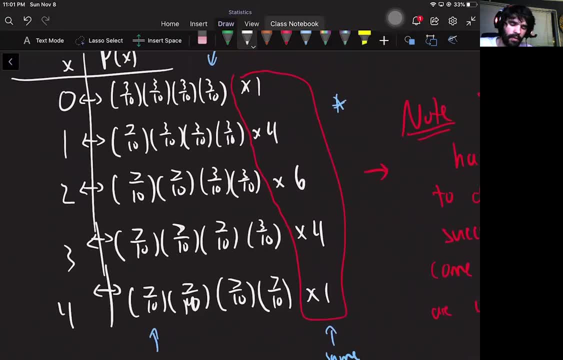 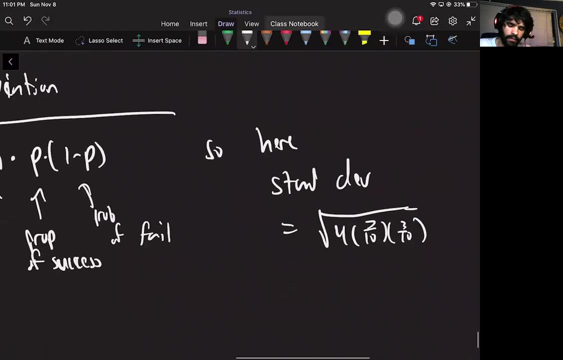 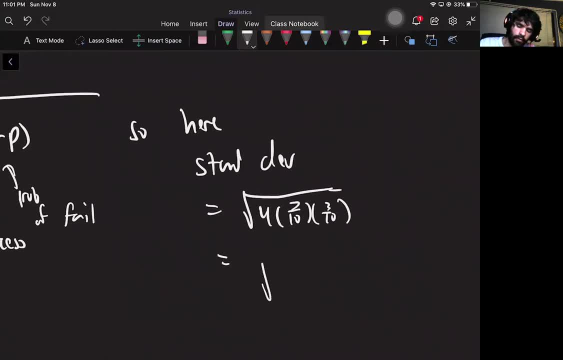 you square them, Then you multiply that probability. All this stuff, Don't wanna do that, Whereas this formula, This is just nice and easy. So B, I think, a four. That's it for this one, this video. I will see you next time.